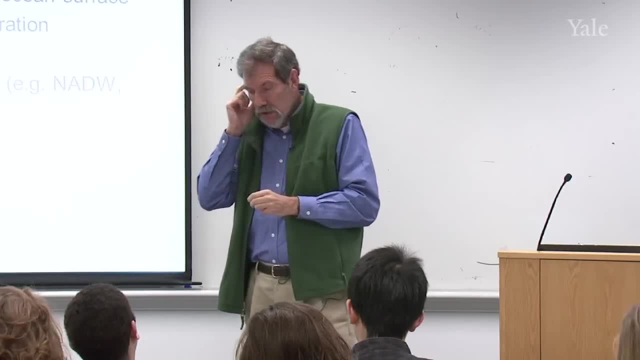 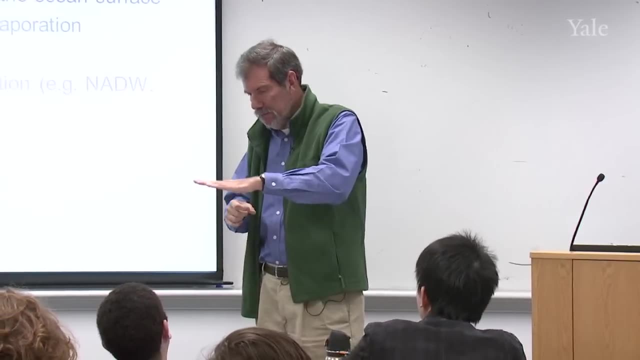 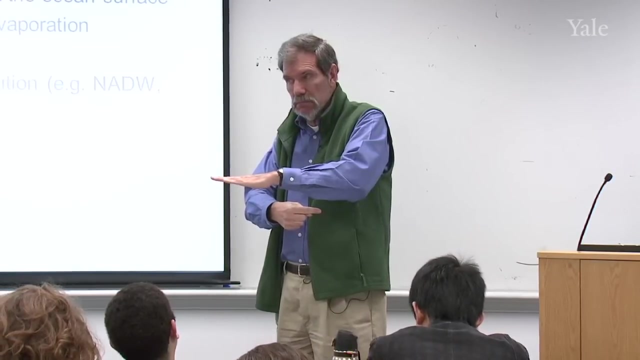 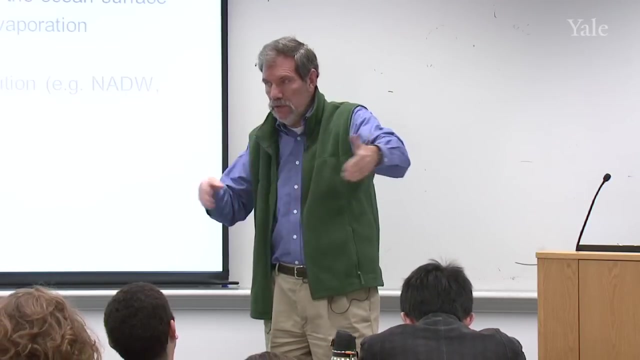 locally by those forcings. In other words, you could have wind blowing from west to east and have, at that same location, wind-driven currents in the opposite direction. For example, these large gyres are driven by the mean wind stresses, westerlies and mid-latitudes, easterlies and 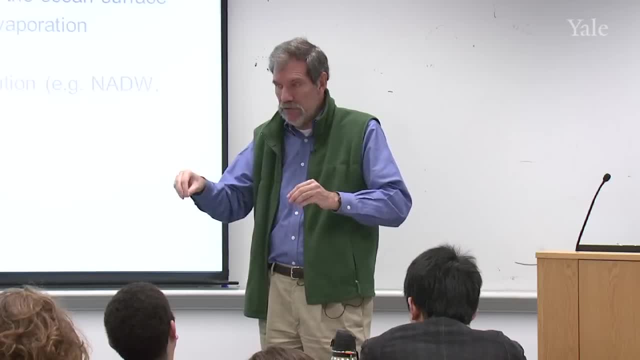 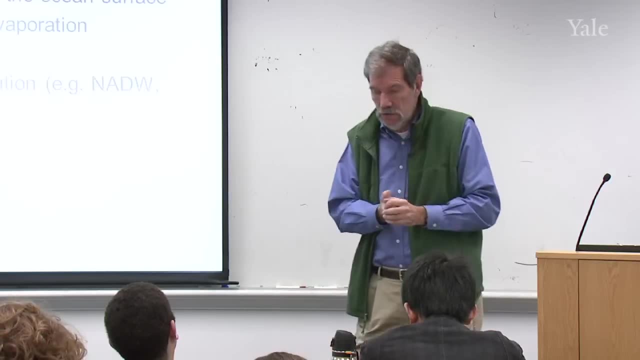 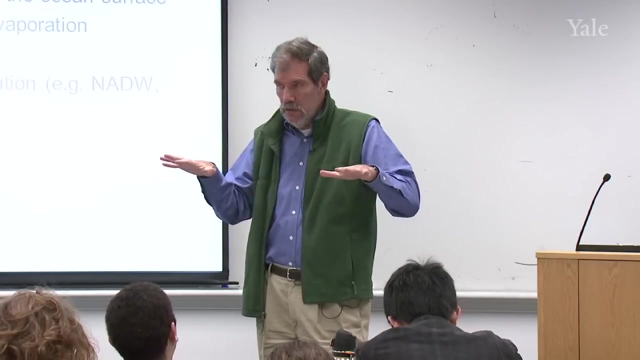 low-latitudes, and there well may be. In fact, there are many places in the ocean where the local wind-driven currents are opposite to the local winds, So don't get confused by that: They're still wind-driven currents. If you turned off, all the wind stresses those currents. 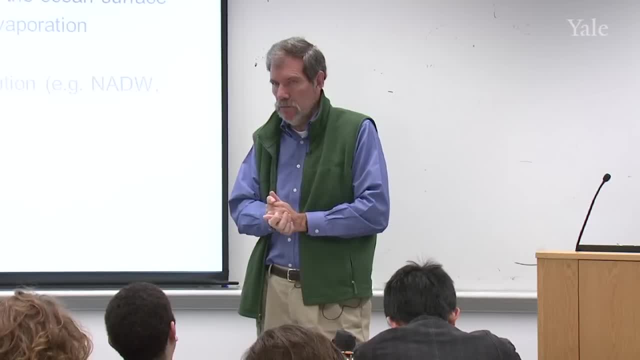 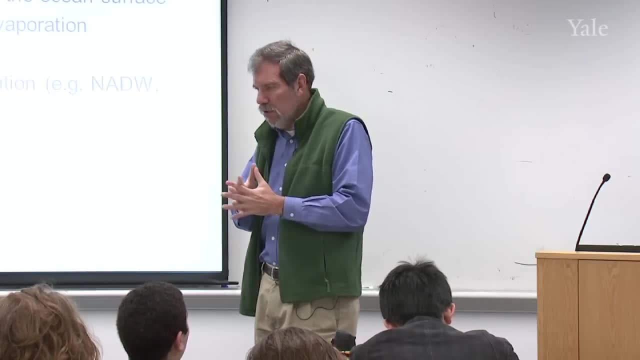 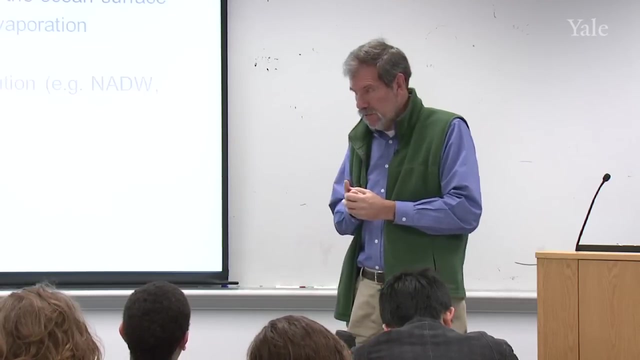 would cease over time. Now, the problem with this nice, clean categorization is that there are some ocean currents that seem seem to be driven by a mix of the two things, For example, the Gulf Stream, which I'll be talking about. 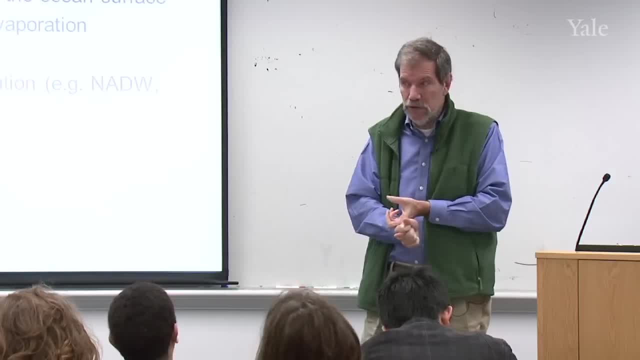 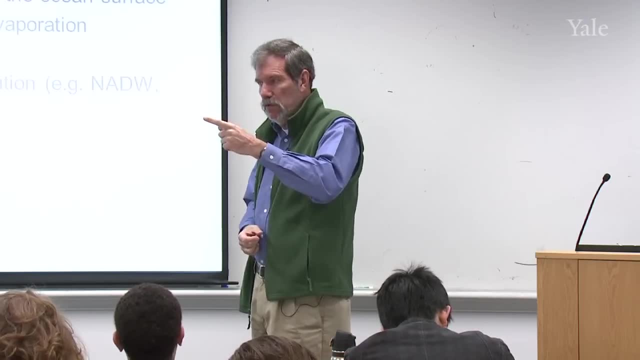 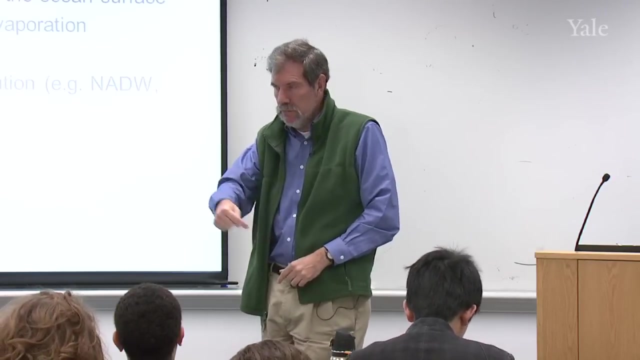 today is generally considered by oceanographers to be a wind-driven current. On the other hand, it carries warm water northward, some of which cools and sinks and returns underneath in the deep ocean towards the south as a colder current. So at that point it seems to be more of a 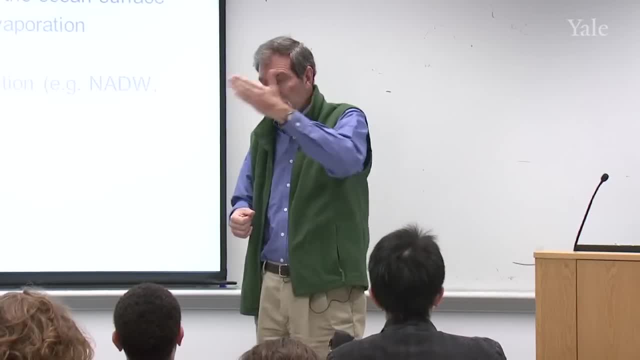 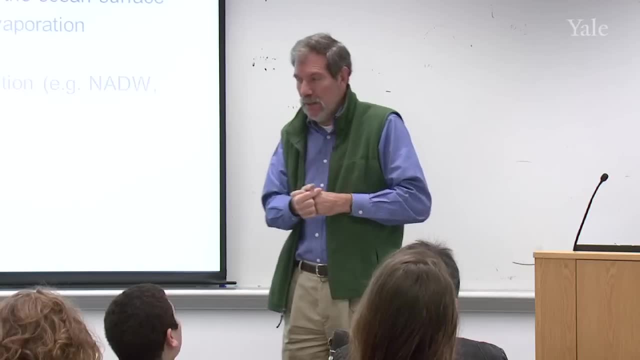 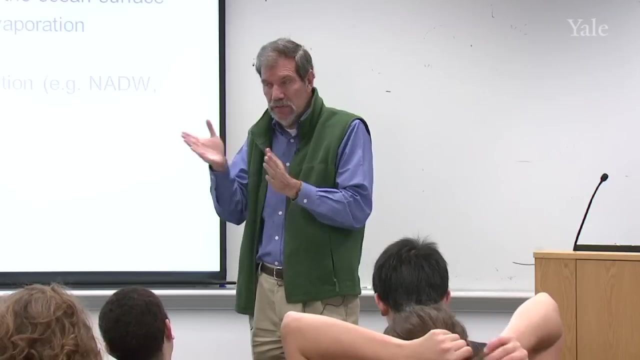 thermohaline current. So some fraction of the Gulf Stream- quote- wind-driven- returns southward as a thermohaline current. So there's an example where we can't quite make that distinction as cleanly as we might like. We just have to live with that though. 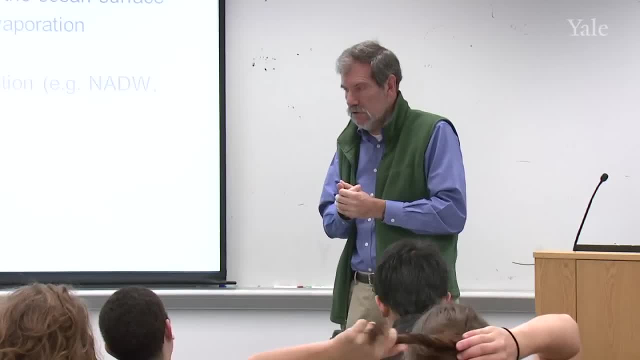 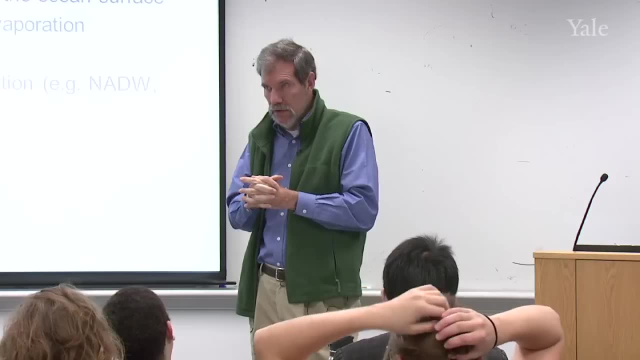 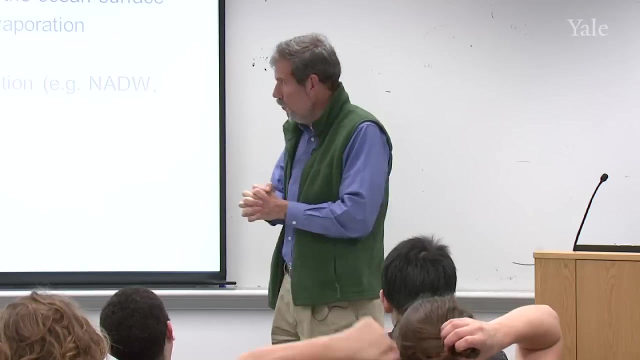 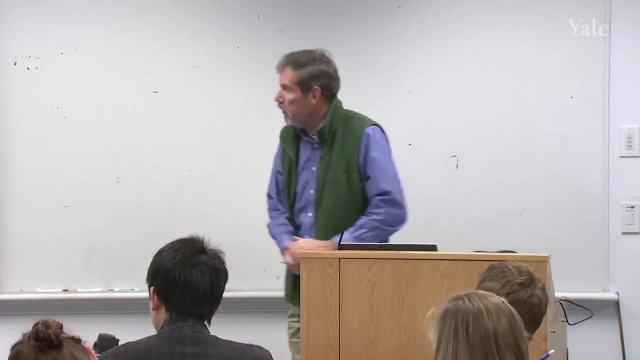 And as our models of ocean currents become more sophisticated, we can try to apply those definitions more and more securely to understanding these differences. Any questions on that? So I'll just back up for a moment or two here and remind you what we talked about with respect to 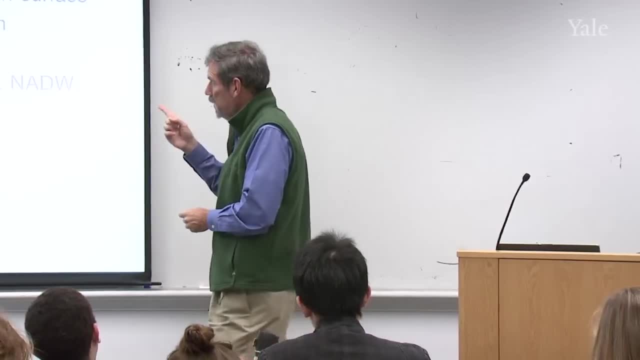 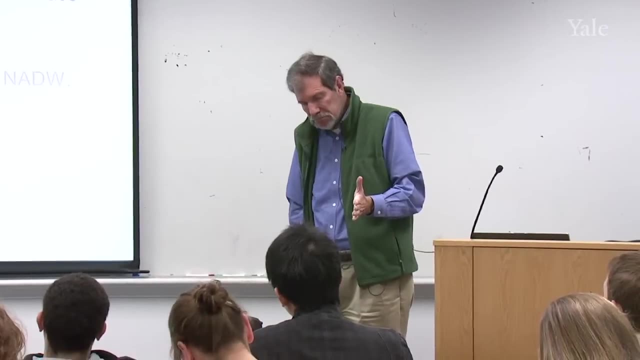 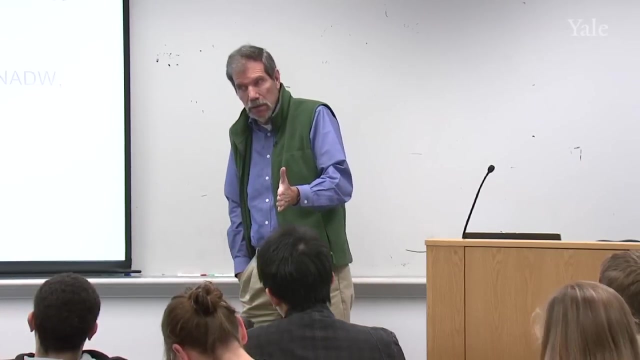 thermohaline circulation. They're driven by density. Typically they tend to be slow currents, probably no more than maybe a couple of centimeters per second, like about this, Maybe even slower In the ocean. So they're quite slow. 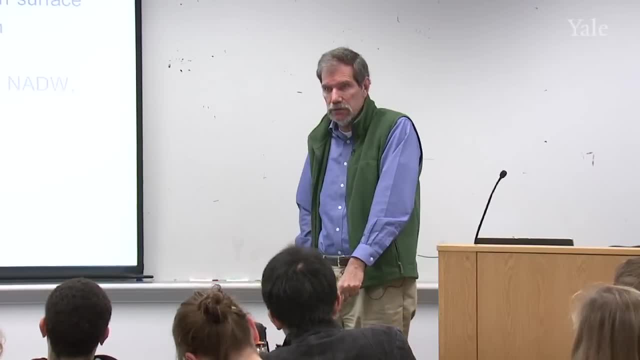 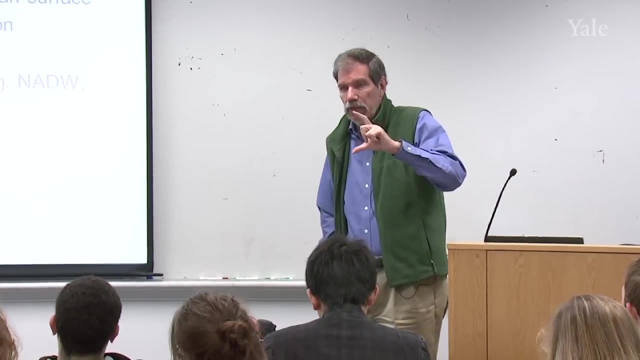 They do, however, extend in some cases right down to the bottom of the ocean, as opposed to wind-driven currents, which are usually in the upper kilometer or so, the upper fifth or so, of the ocean column. They're responsible for the water mass distributions. 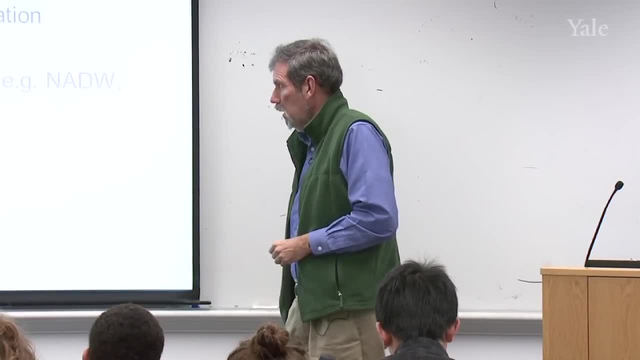 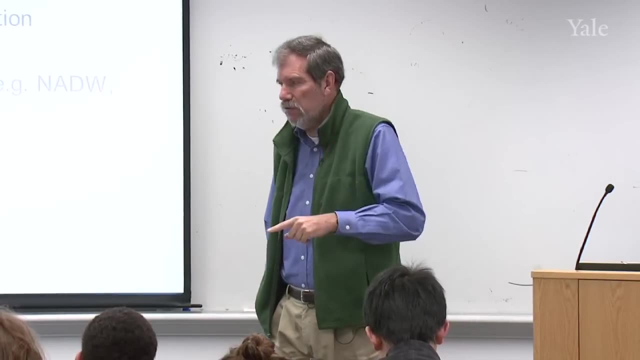 We talked about the ones in the Atlantic Ocean, That conveyor belt circulation between the Pacific and the Atlantic Ocean and these estuaries and you know the inverse estuary circulations are all thermohaline circulations. We talked about that. 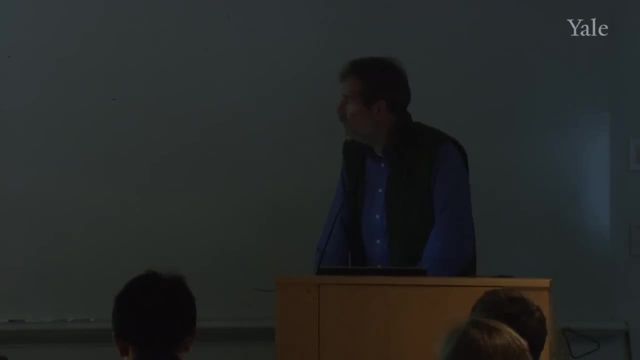 Stop me if you have any questions on these sections. We went over them before. That was a north-south section for temperature in the Atlantic, for salinity in the Atlantic. Oh, I didn't mention one thing that probably should be discussed. 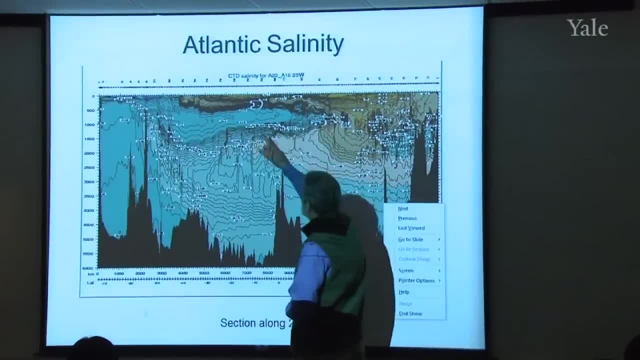 There's this thing called the thermohaline circulation. There's this thing called the thermohaline circulation. There's this thing called the thermohaline circulation. There's this blob of salty water. You'd expect the water in the tropics and subtropics to be. 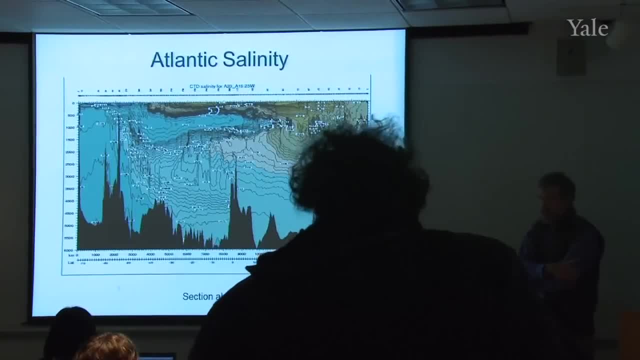 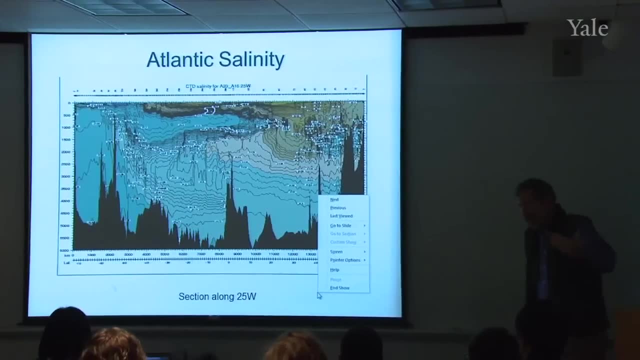 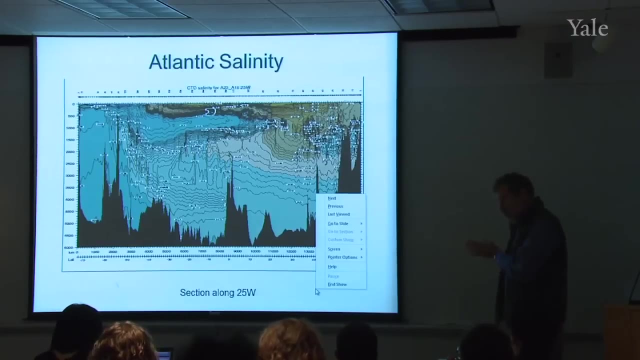 salty because there's an excess of evaporation at the surface of the ocean. But what explains this blob of salty water is actually that outflow from the Mediterranean Sea. that salty outflow from the Mediterranean Sea then moves westward across the Atlantic Ocean and catches us in this north-south section. So this blob of salty water. you'd expect the water in the tropics and subtropics to be salty because there's an excess of evaporation at the surface of the oceana. But what explains this blob of salty water is actually that outflow from the Mediterranean Sea then moves westward across the Atlantic Ocean, then catches us in this north-south section, etc. 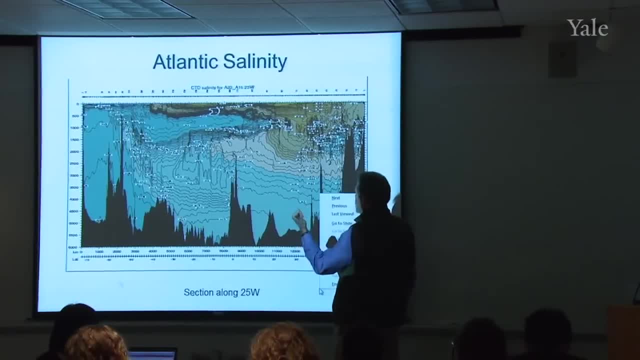 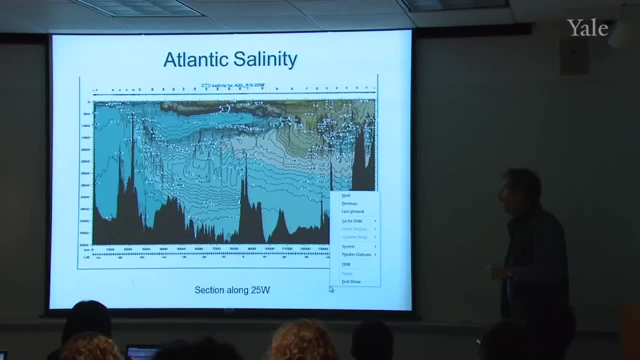 If that's north and that's south, then that's west and that's east. This is the Mediterranean water coming into the section from the east as an outflow from the Mediterranean, So it flows over the Sill there in the Straits of Gibraltar. 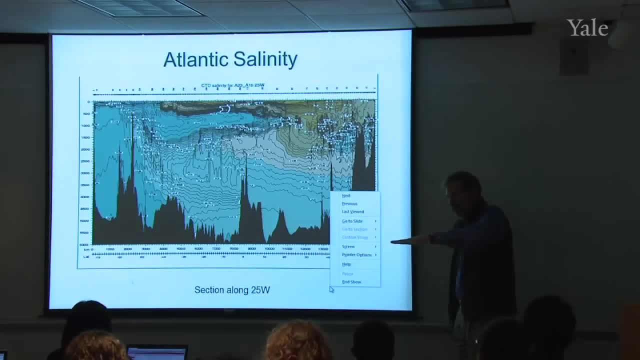 Flows down until it finds its appropriate density level. where the water above it is less dense, The water below it is more dense, And then it floats horizontally as a tongue of salty water, finally reaching that section. It's part of the reason why the North Atlantic deep water 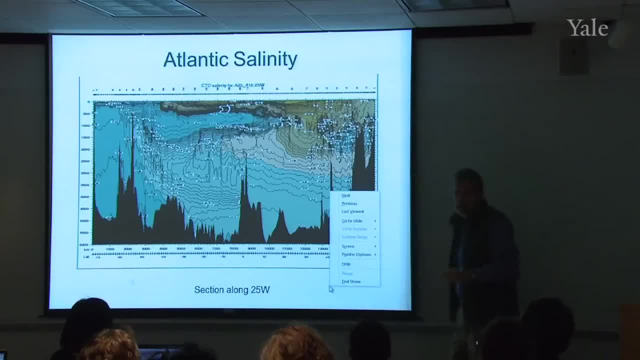 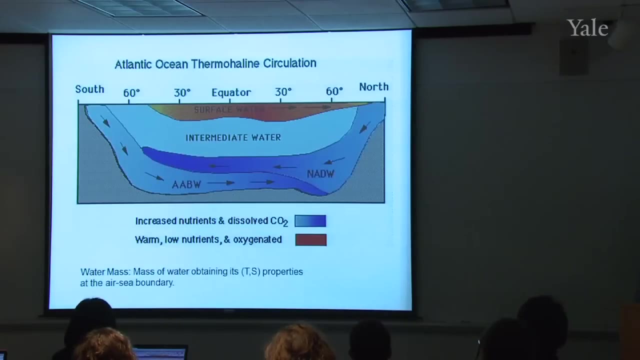 is generally salty because the Mediterranean water gets entrained into that North Atlantic deep water. We talked about the oxygen And this was the summary, in a north-south section of the Atlantic Ocean, thermohaline circulation. Any questions on this? So this is the Antarctic intermedial water, the North 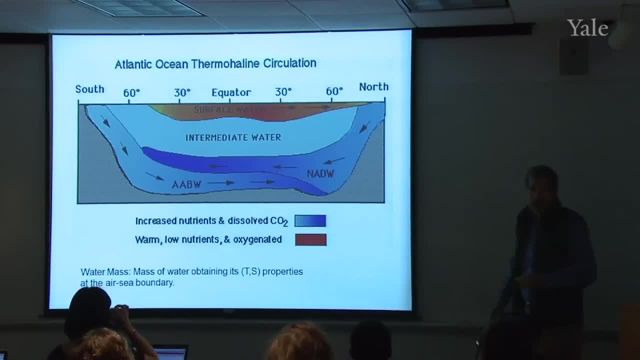 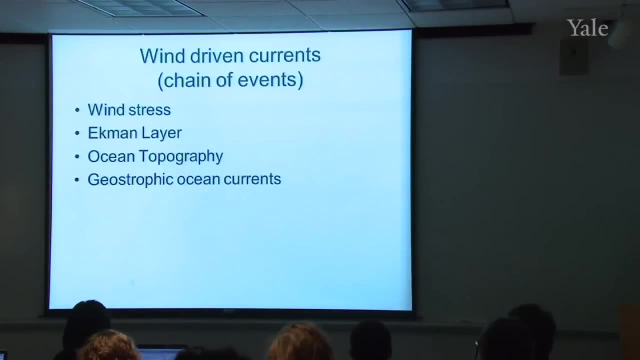 Atlantic deep water and the Antarctic bottom water. We talked about this. OK, now I got into wind-driven currents a bit. I want to review that as well. The chain of events, as we understand it today, is that the wind stress produces. 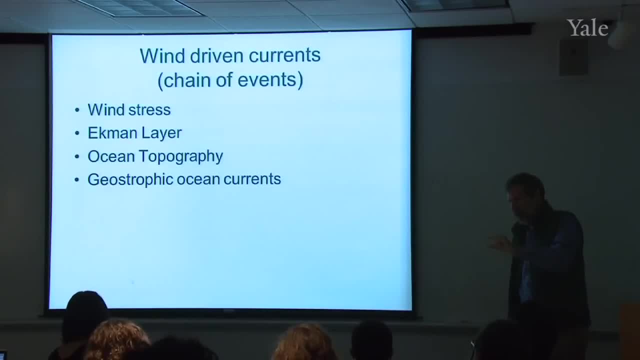 It produces a shallow transport of water in the layer that feels that wind stress directly. That's a pretty shallow layer, probably only 100 meters deep, And in that layer the water gets pushed off to the right of the wind stress in the northern hemisphere. 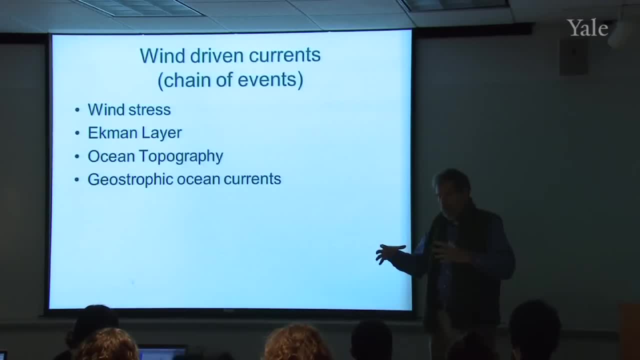 That Ekman layer transport piles up water- for example, in the middle of the North Atlantic gyre There's a piling up of Ekman layer drift- And that in turn, that slight non-uniformity in the height of the ocean surface generates pressure gradients beneath. 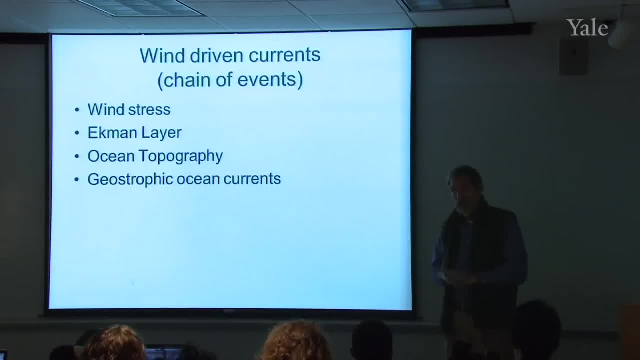 horizontal pressure gradients that then generate geostrophic ocean currents. I mentioned that we can now measure this, and I'll show you that plot again in just a moment, But it dawned on me that I forgot to mention that there were clues to this. 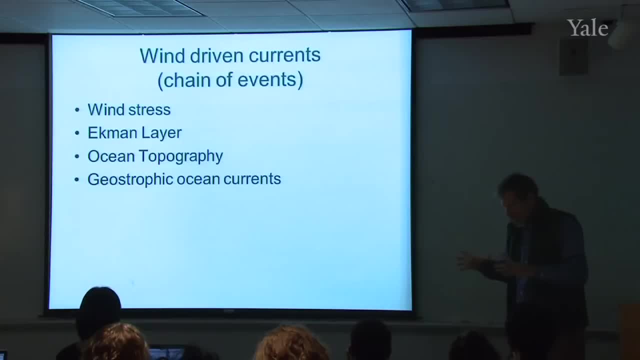 Even in the early 1800s, Even in the early days. For example, the center of the North Atlantic gyre is referred to as the Sargasso Sea. Does anyone know where that term, Sargasso Sea, comes from? It's an old term. It goes back several hundred years. If you take a ship across the Atlantic, through the middle of this gyre, when you get into that region of the ocean you begin to see floating pockets of water, Pockets of plant material. It's mostly Sargassum weed. 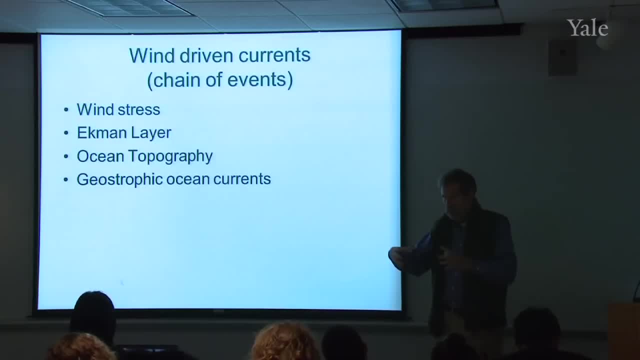 It's floating there And the reason why it's collected there is because of the Ekman currents pushing it there. So we had some clue that that was a region of convergence even before we could measure that sea surface height anomaly from satellites, If you dumped in. and now that there's more pollution in the 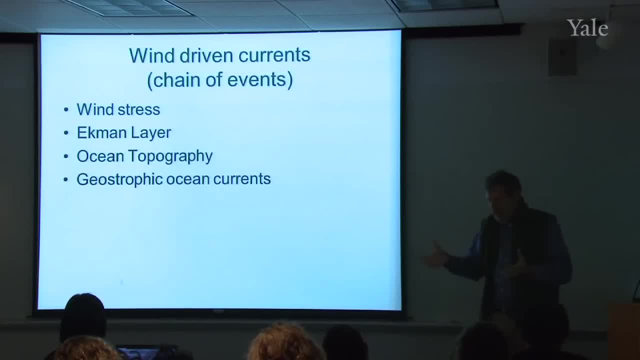 ocean. people are going to say: well, that's not good. People have dumped loads of trash into the ocean that floats. Some of that is found in the Sargasso Sea as well. It's just an area where water tends to collect and then of. 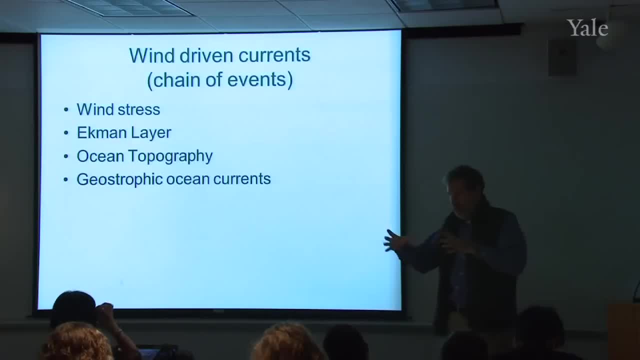 course sink eventually. But in the collecting all the things that float remain kind of gathered there in the middle of the ocean. We've also found these gatherings in the middle of the other ocean gyres. So there's evidence that ocean water does collect there and 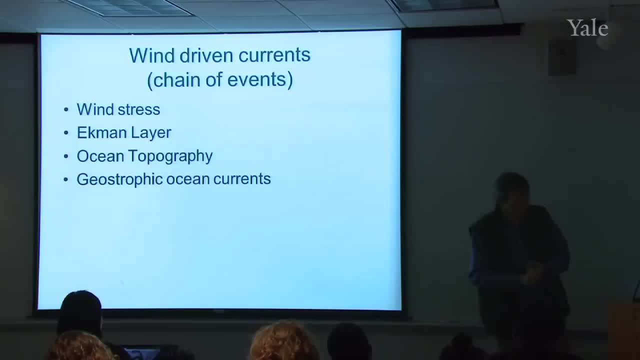 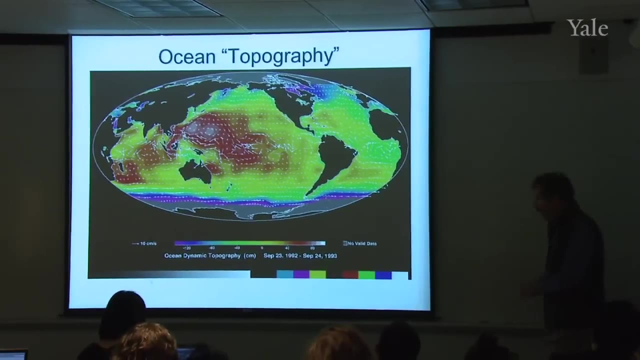 the things that float are still found there. So the fact that it's called the Sargasso Sea gives another clue to this sequence of events. So there's the winds and there's the ocean. topography as measured from space with units in centimeters. 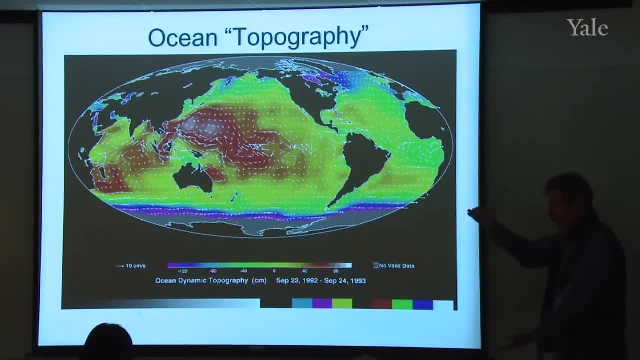 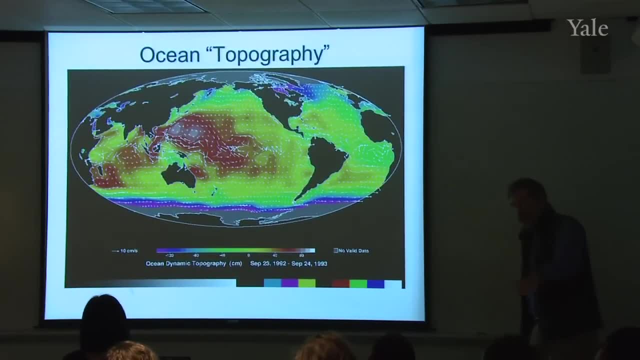 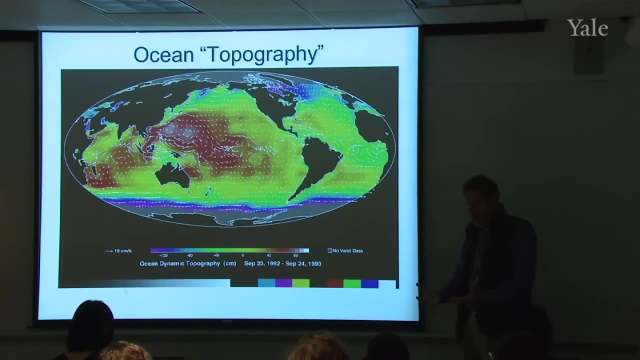 Typically it's only a topography of about like this: You would never notice it if you were sailing through there, But the water is slight. It's slightly higher there than the geoid of the Earth. There's a surface you can imagine, nearly a sphere, which. 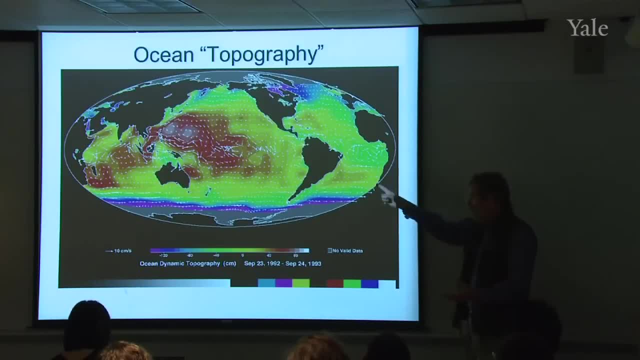 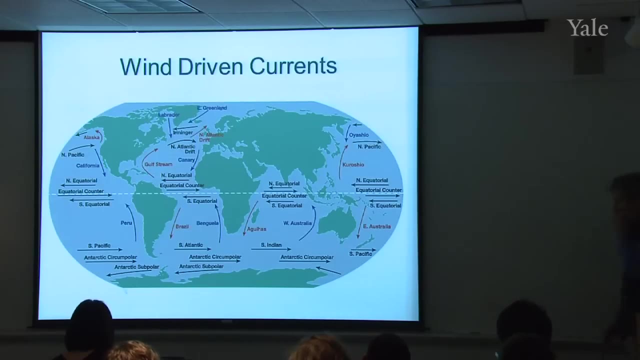 we consider to be the level surface, And this rises slightly above that level surface and then, in turn, gives rise to the pressure gradients underneath that, And these are the wind-driven currents. I don't want you to think that you're going to be able to do. 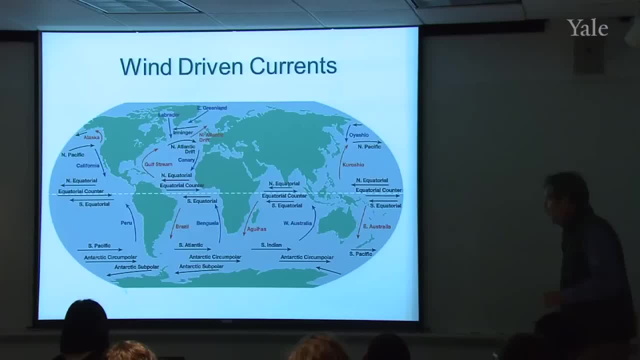 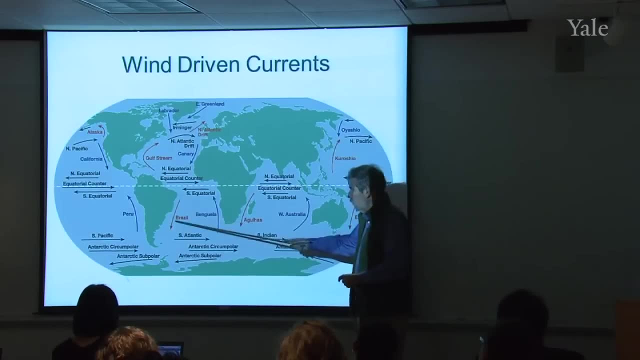 all these things. I don't want you to memorize all these names, except some of them probably should be known, And some of them are quite obvious that it's hard, once you've seen them, not to know them. For example, the Brazil current runs down the coast of Brazil. 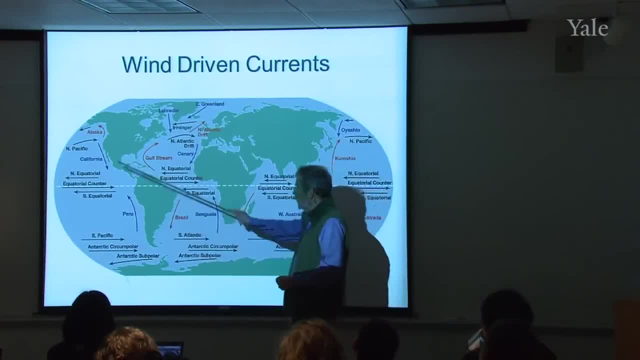 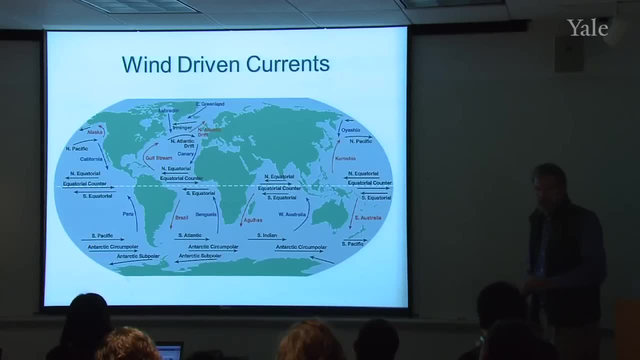 The Peru current runs up the coast of Peru. The California current, the Alaska current, the West Australian current, the East Australian current- Pretty hard to forget those once you've seen them. The Gulf Stream is part of the North Atlantic Gingrich, The North Atlantic Gyre. the word gyre is spelled G-Y-R-E. and it refers to these circular current systems forced to be circular because the continents prevent them from going all the way around the Earth. Only in the Southern Ocean, where you get the Antarctic circumpolar current, do you get a current going all the way. 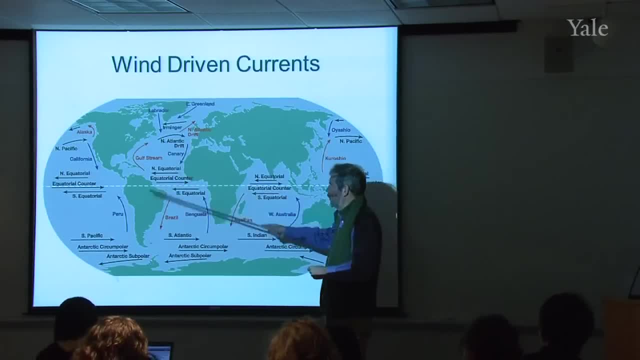 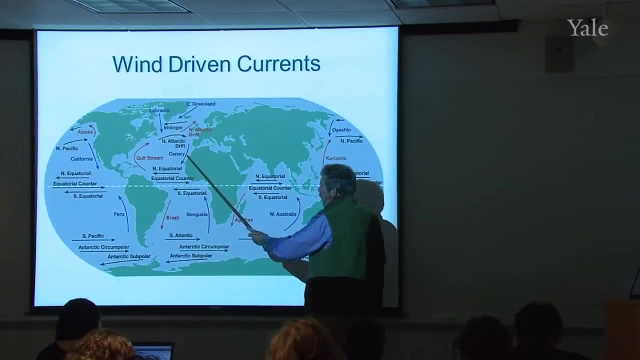 around the ocean. Otherwise, the continents break up these wind-driven currents into gyres: The North Atlantic Gingrich. The North Atlantic Gyre consists of the Gulf Stream, the North Atlantic Drift, the Canary Current and the North Equatorial Current. Some of the Gulf Stream ever breaks off and becomes the North Atlantic Drift, which eventually goes in to the Arctic Ocean. You can have reverse currents in the very high latitudes, like the Alaska Current. Notice that goes opposite to the main North Pacific Gyre. 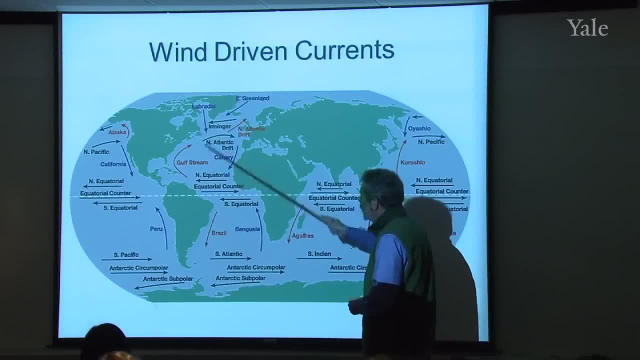 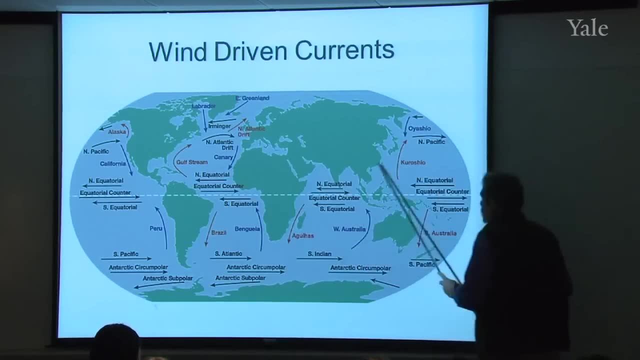 And the Labrador Current in a sense is the North Atlantic Gyre and in a sense goes a little bit opposite to the North Atlantic Gyre as well. The equivalent to the Gulf Stream in the Pacific Ocean is the Kuroshio Current. 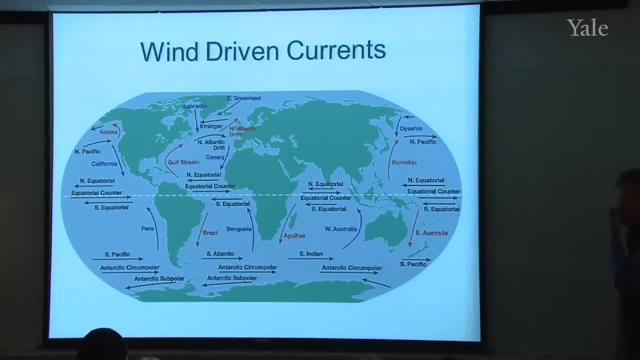 And there's a lot of studies kind of comparing those two currents because they play the equivalent role in the two large Northern Hemisphere basins. They're both warm currents and you can find equivalent things in the Southern Hemisphere as well, the three warm currents. 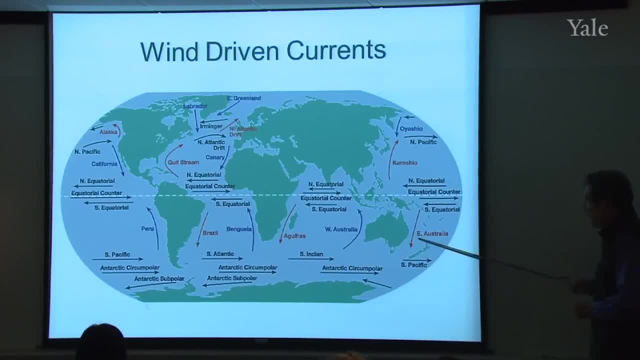 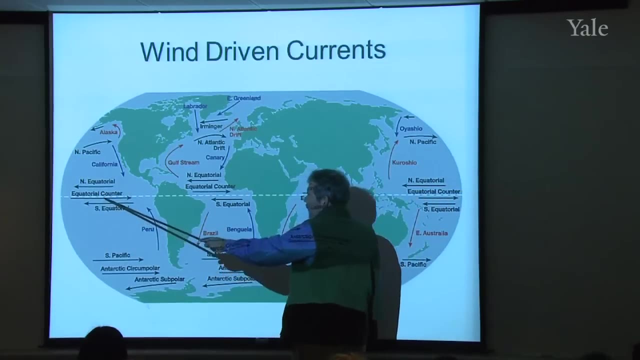 Would be the Brazil Current, the Alguas Current and the East Australian Current, each returning equatorially warmed water down into the high latitude, colder areas Near the equator. things can get pretty complicated. You can have an equatorial countercurrent. 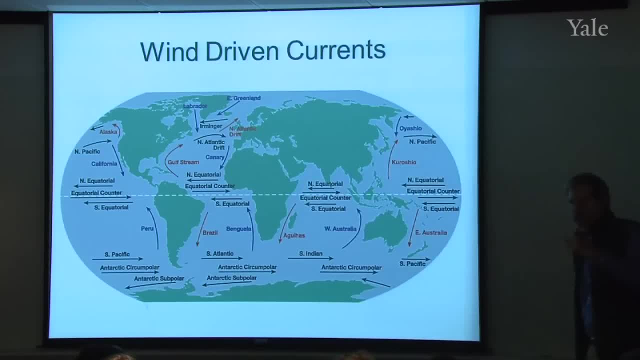 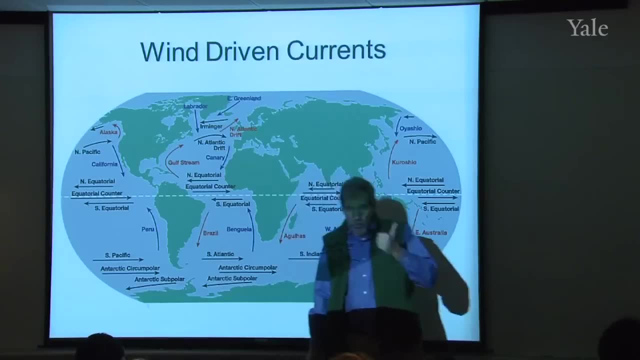 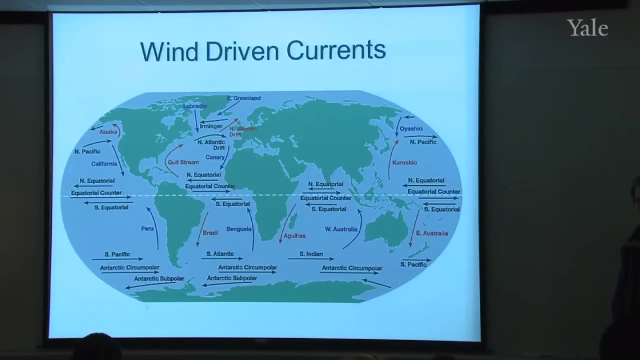 And notice that this would be the region of the trade winds blowing from east to west. And yet there's the countercurrent, a wind-driven current, I propose to you, And yet it's running opposite to the local wind direction. So that's one of those confusing points where the 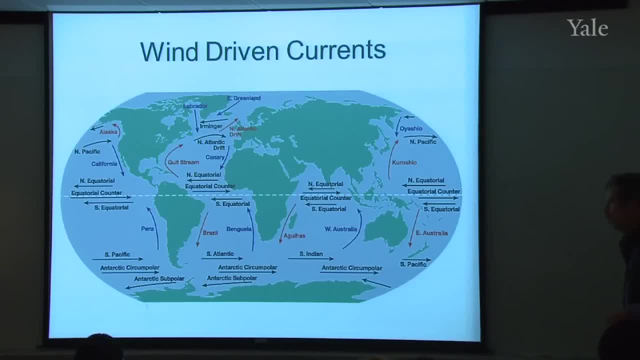 winds don't always seem to be pushing the currents around locally, But then again that has to do with this indirect effect. It's not just the wind blowing on the water to make it move. You've got that chain of events: The Ekman layer, the piling up of the water, and then the 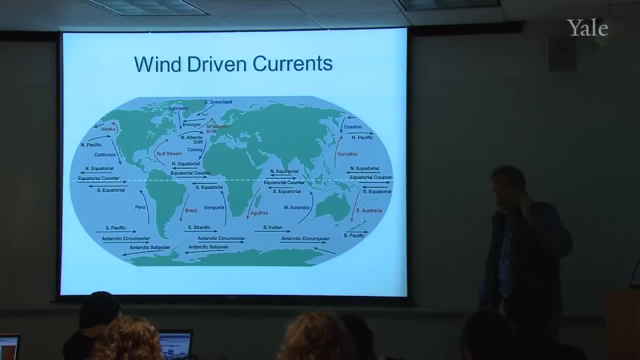 geostrophic currents. It's not a direct air pushes water, water moves scenario. It's a little more complicated than that. Another interesting fact, which is why we have to have this slightly more complex theory, is that these ocean currents, for the most part, do extend about a kilometer. 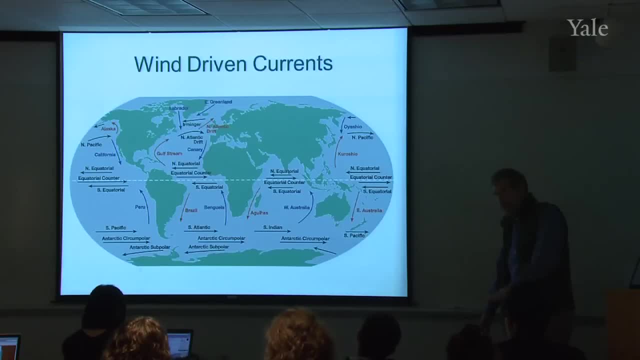 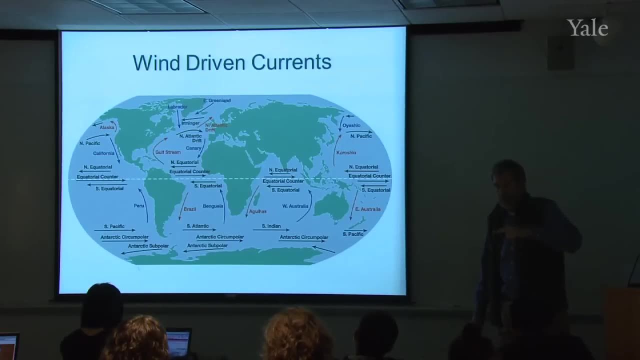 down into the ocean. They don't extend to the bottom, but they extend about a kilometer down, and that's far deeper than the wind stresses felt directly. So in order to explain that, we have to have this more complicated theory, Then it's the pressure gradients which extend down to. 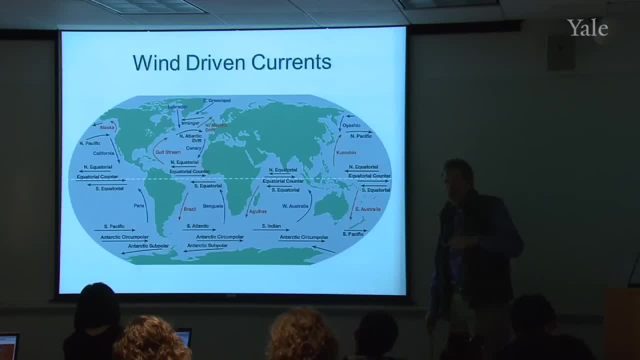 about a kilometer below the surface that are generating these so-called wind-driven currents. When I say they're geostrophically driven or geostrophically balanced, I mean they have a balance between pressure gradients. If it's pressure gradient force and Coriolis force, where 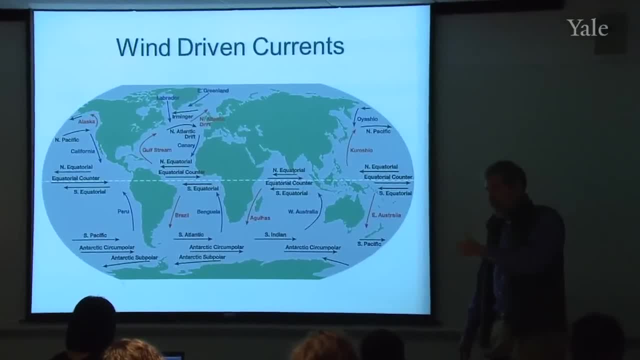 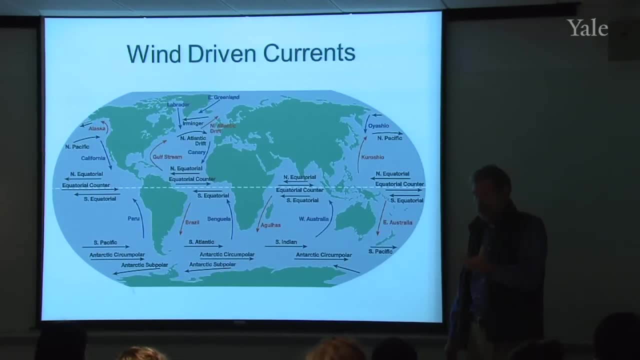 does wind appear then? in that, If it's Coriolis force and pressure gradient force, does that mean wind is not active? No, Wind was important in setting up the pressure gradient force, so wind is still in there, even though it doesn't. 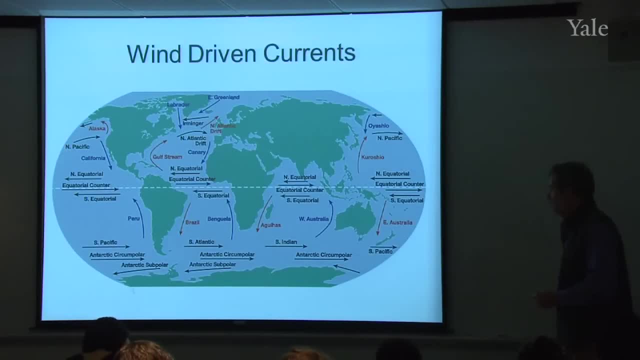 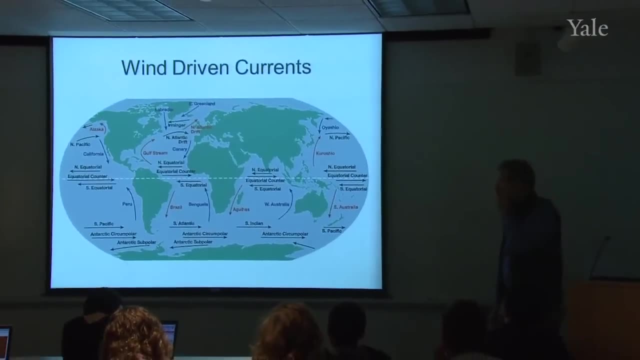 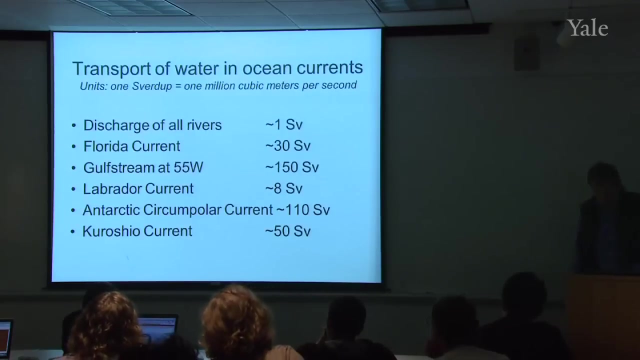 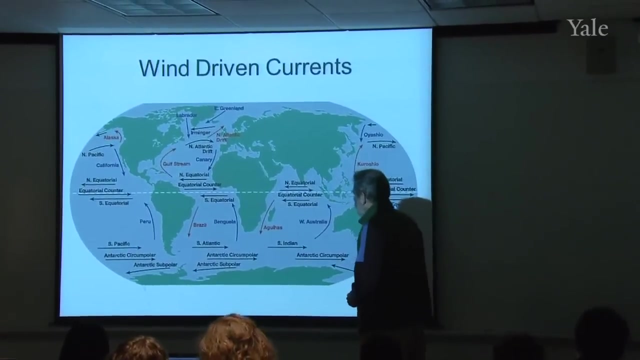 appear directly in that force balance. Any questions on this current map of the world? OK, now we try to estimate how much water is moving in each of these currents. Now, in some cases it's easy to do, For example, where the Antarctic circumpolar current. 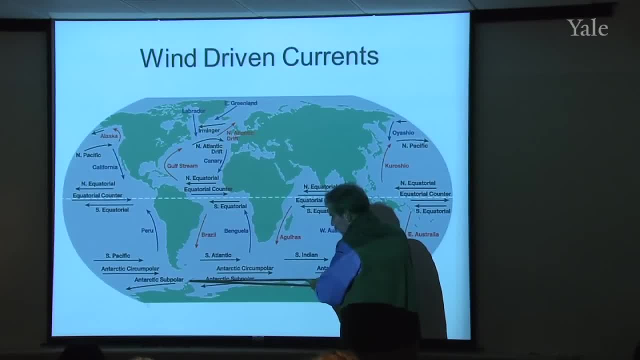 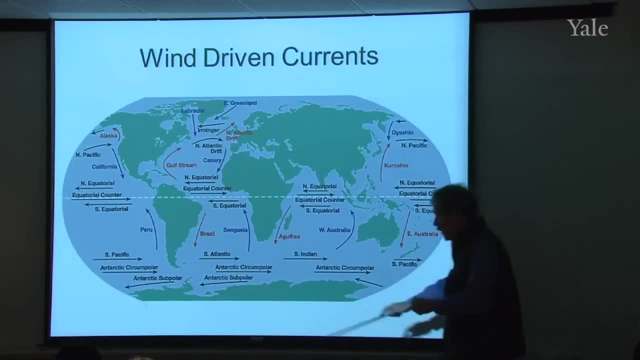 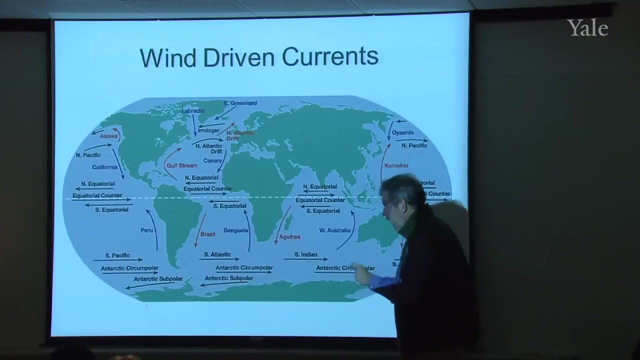 passes through the Drake Passage between the Antarctic Peninsula and the southern tip of South America. that's a well-defined channel, if you like, And so we can measure with ships and so on and current meters We can measure how much water flows between there and that. 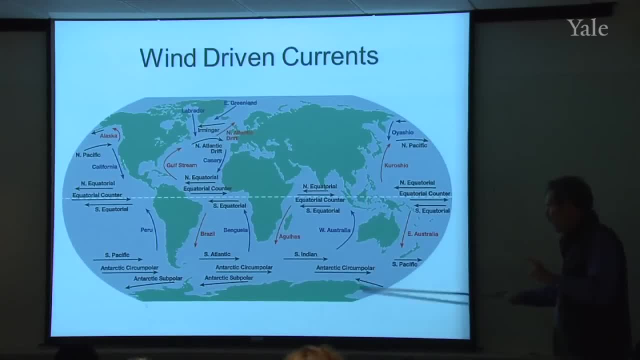 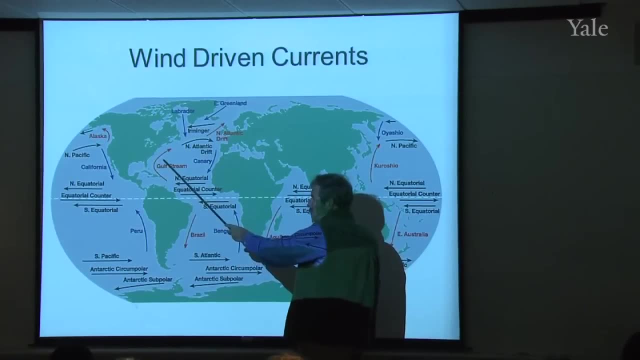 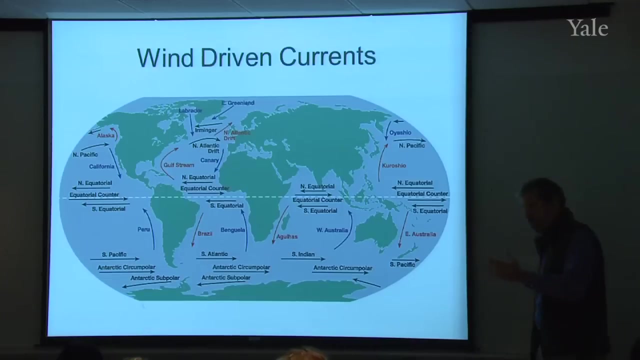 would be a local measurement of the Antarctic circumpolar current In other places, for example the Gulf Stream. where do you put the outer edge? OK, it does weaken as you go out, as I'll show you in a minute, but it's still a little bit ambiguous about. 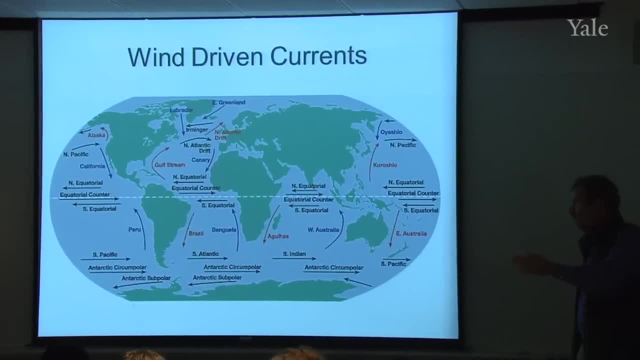 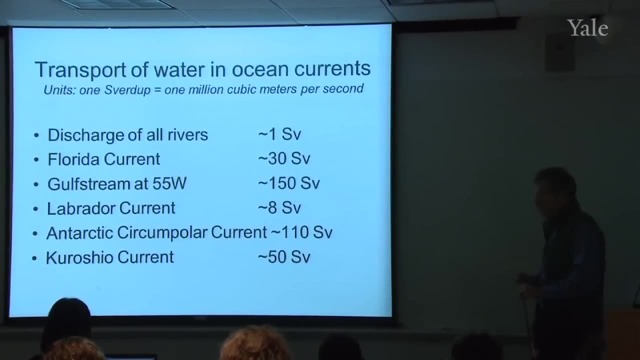 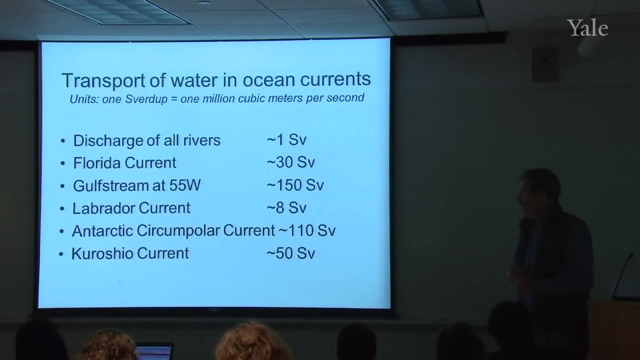 where you mark the outer edge of the Gulf Stream. Nonetheless, we have come up with these estimates for the ocean currents, and this isn't inclusive, but it's a few examples of estimates of how much discharge are in some of the major ocean currents around the world. 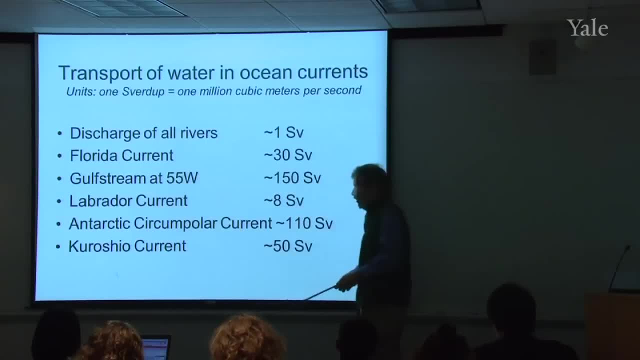 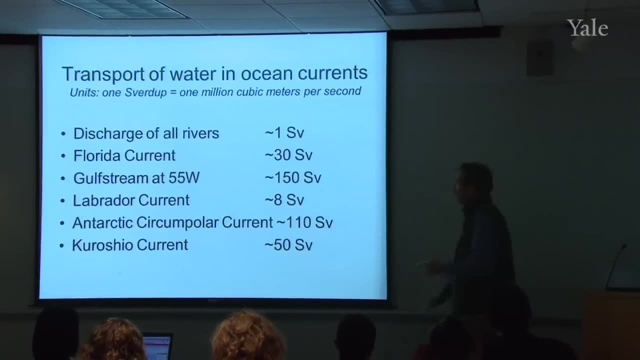 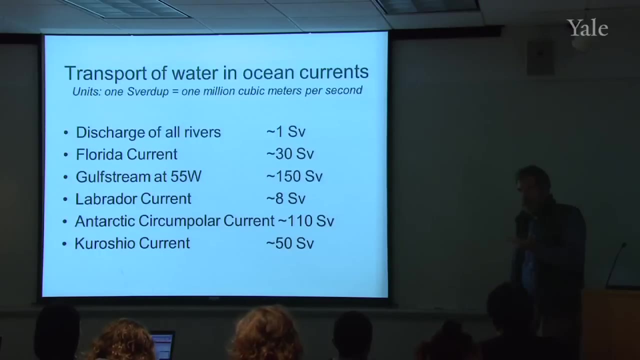 And we're using the unit of Spherdrop here, which is named after a famous oceanographer. It's not really an SI unit, but it's closely related to one. it's simply one million cubic meters per second, So it's a volumetric discharge rate. 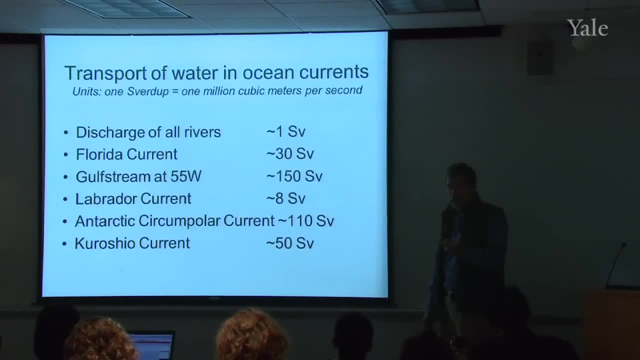 Just like we've been using in rivers. It's a million cubic meters per second. And one way to remember this: that if you add up all the discharge of rivers in the world, all the freshwater rivers dumping water into the ocean, the number is 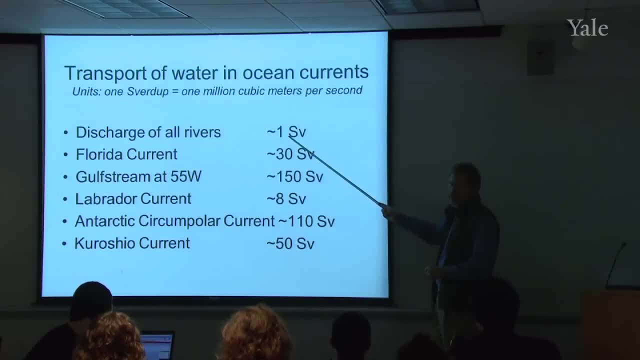 approximately one Spherdrop. It just turns out by accident to be that way, So it's easy to remember. summing up: the Amazon, the Mississippi, all the major rivers, the amount of discharge, the amount of discharge. You get a number, something like this: 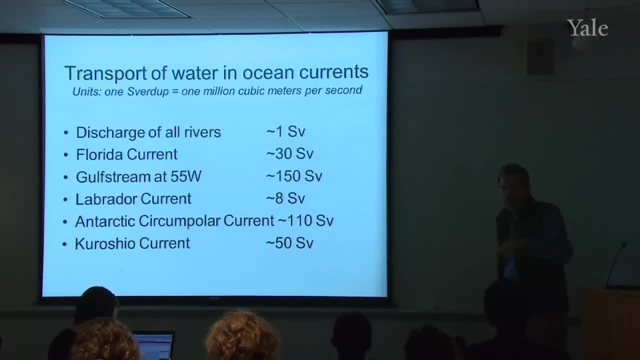 It's a good comparison point for then looking at the discharge in the ocean currents, The Florida Current, which is where the Gulf Stream is passing up along the coast of Florida. it's only 30 Spherdrops there, but a few hundred miles north of there. 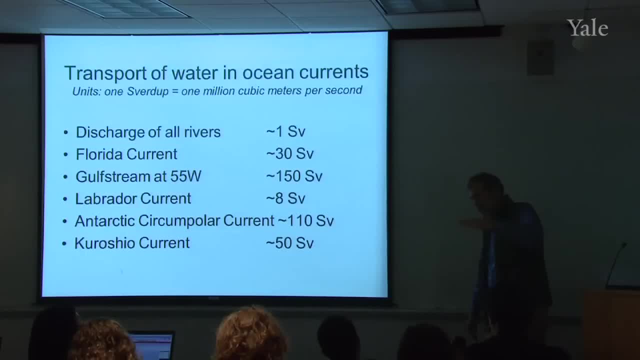 where it's, just leaving Cape Hatteras and heading eastward. if you do a north-south section through it, it's grown to 150 Spherdrops, One of the strongest currents in the world, The Labrador Current, that cold current coming down. 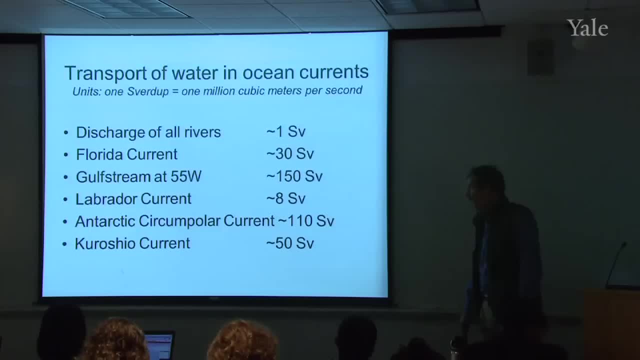 through the Gulf of Maine and reaching in some cases even Massachusetts, has about eight Spherdrops. That Antarctic Circumpolar Current that I mentioned, at least where it passes through the Drake Passage, is 110 Spherdrops and the Corotio Current is 50 Spherdrops. 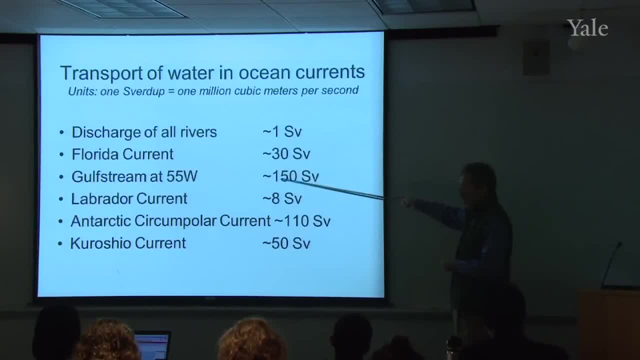 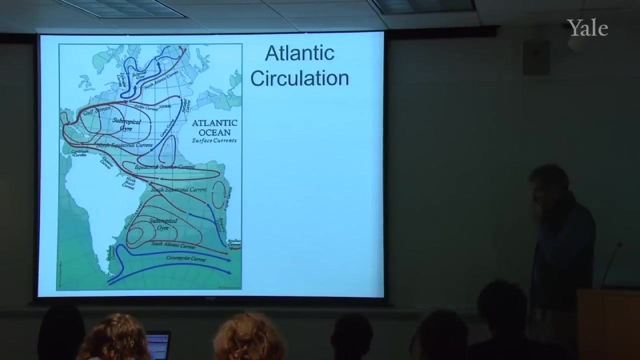 somewhere between these two estimates for the Gulf Stream. These are just round numbers, but they'll give you some sense for how much water is moving around in these ocean currents. So let's focus on the Atlantic Ocean for a few minutes. It's complicated. 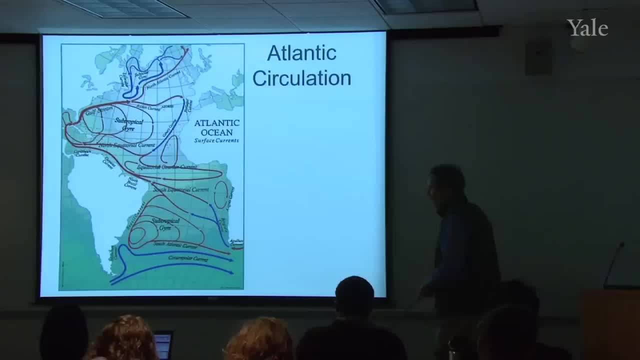 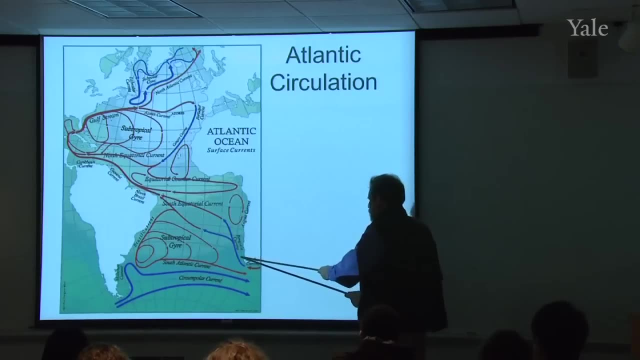 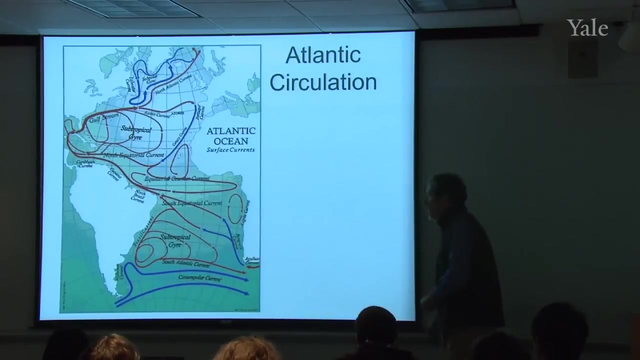 The Antarctic Circumpolar Current flows along. at the southern edge of it, Some cold water gets peeled off and put northwards into the Benguela Current, And we've talked about that. We've talked about the role that this place plays in keeping the South Equatorial Atlantic rather cool. 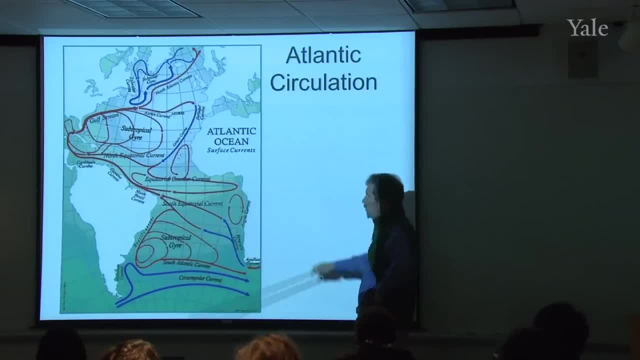 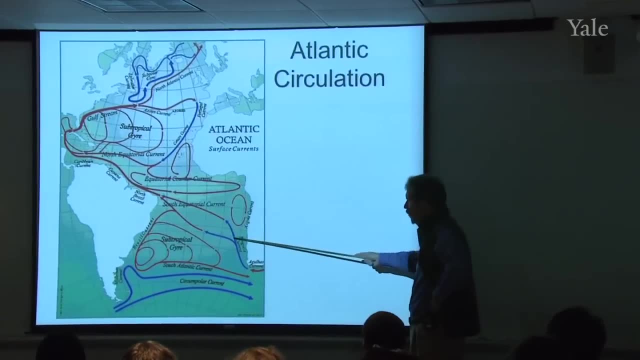 Very few hurricanes form in here and the ICCZ never really shifts south of the equator in this ocean, and that's because of the cold water being brought up by the Benguela Current. There is a South Pacific- sorry, a South Atlantic Gyre. 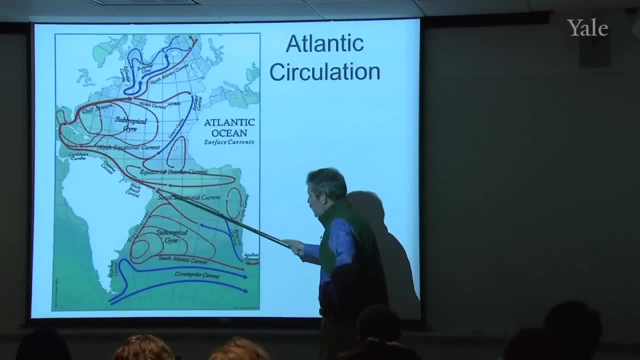 and it consists of the South Equatorial Current, the Brazil Current, the South Atlantic Current And then the return in the Benguela Current. The equatorial region, the equator is here. It's a little complicated. There are some counter currents. 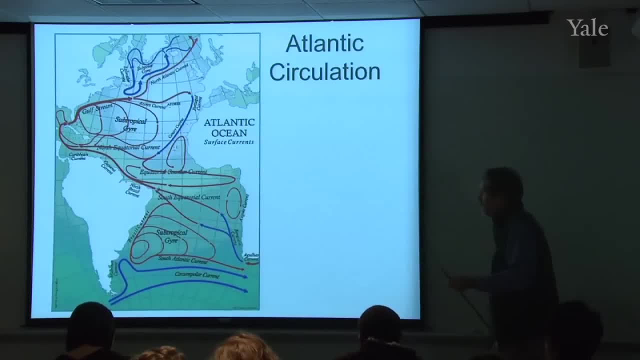 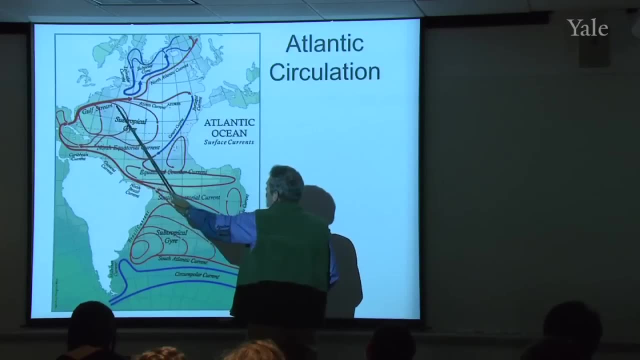 So let's shift up into the northern hemisphere, where I'll spend most of my time here, And that is. you've got another gyre, a subtropical gyre consisting of the Gulf Stream. Some would call this the Gulf Stream Extension, or the North. 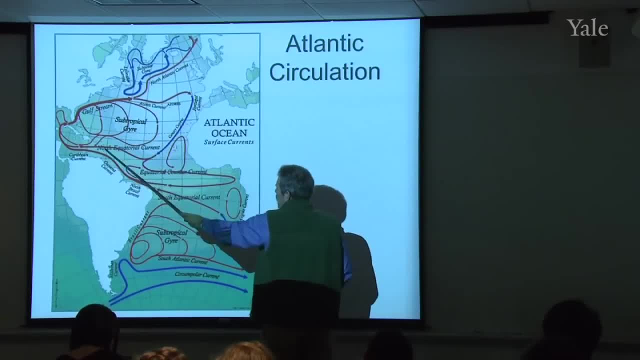 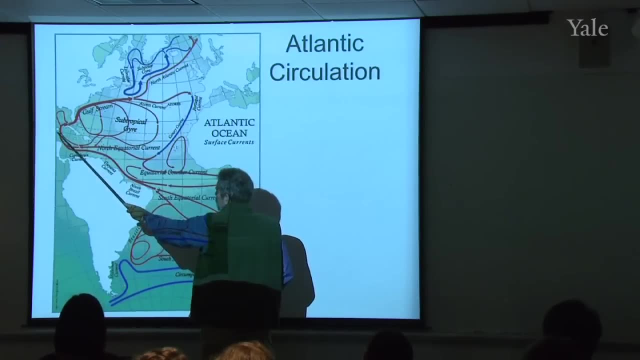 Atlantic Current It returns in the Canary Current and then the North Equatorial Current. there Some of this enters into the Caribbean Sea. Then between Mexico and Cuba it flows up into the Gulf of Mexico, then comes out right along the coast of Florida. 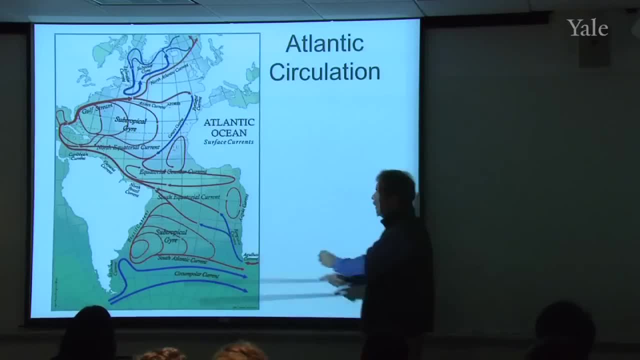 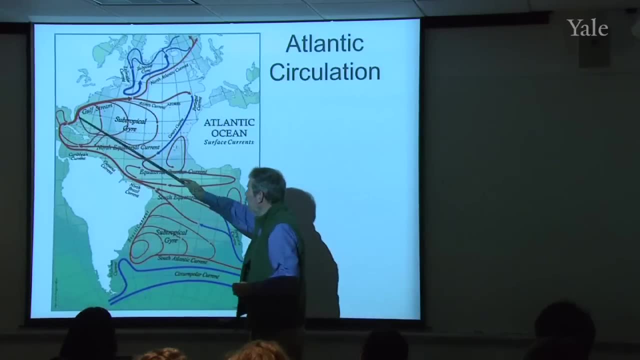 And that's the number I quoted you for the Florida Current. But then additional water joins it and by the time it gets out here it has more total transport than it has in the Gulf as it moved up along the coast of Florida. 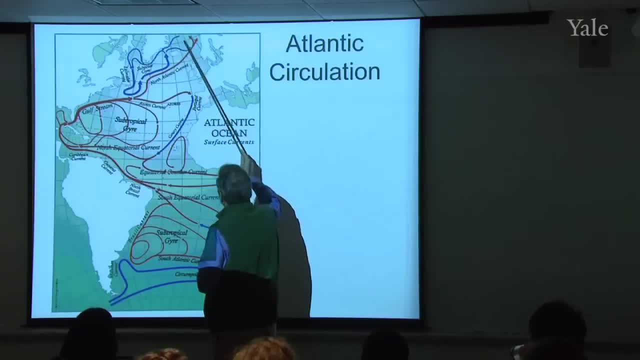 Oh, then you've got the Labrador Current up here. Water coming down out of the Arctic Ocean moves along the east coast of Greenland, back up along the west coast in Baffin Bay and then becomes the Labrador Current and comes down here. 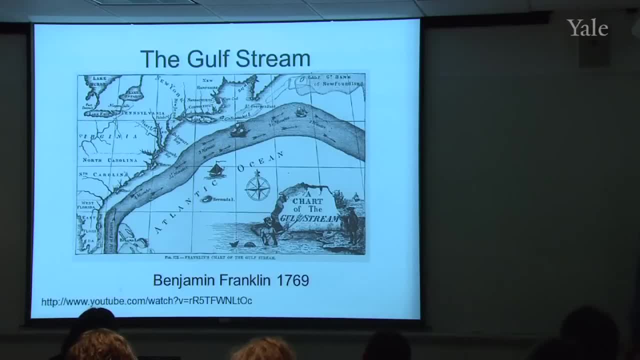 And that's a cold current. So the Gulf Stream was discovered. well, it was known, in a way, from the earliest sailing expeditions across the Atlantic Ocean, But actually it was Ben Franklin who did the first scientific study of it. 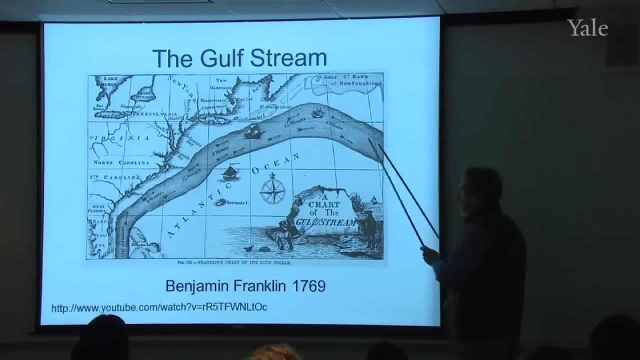 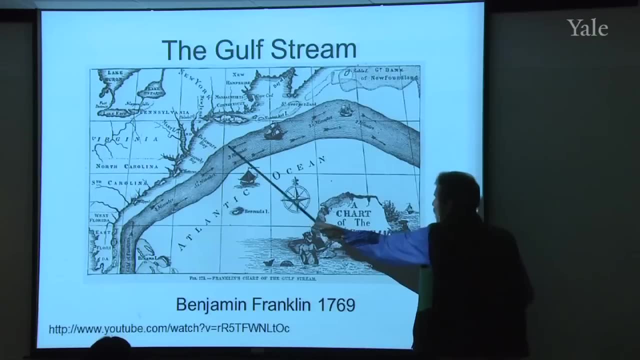 By looking at ships' logs. he himself took that trip a couple of times when he was posted as being ambassador to the French court, And he would take observations as he traveled across, And this is his map from approximately 1769.. We'll compare that with what we know today about the. 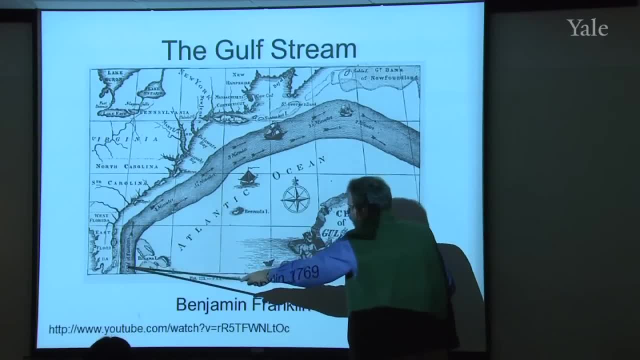 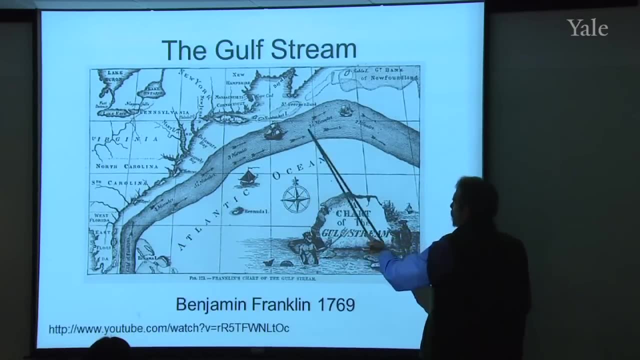 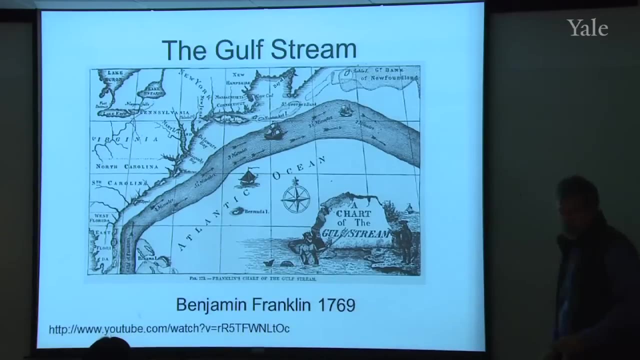 about it, but he's got the basic idea right. It comes up along the coast of Florida to the Cape Hatteras and then seems to leave the coast and move out towards the east and doesn't come that close to us here in Connecticut. we're right there. 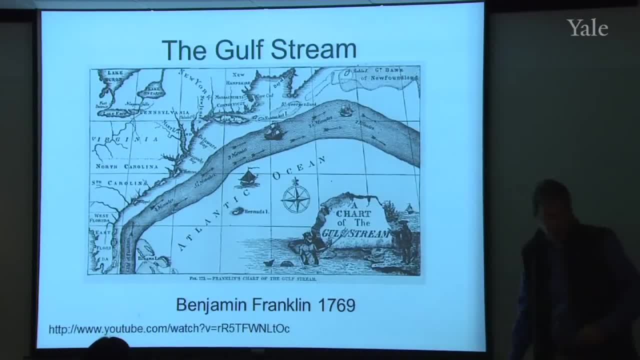 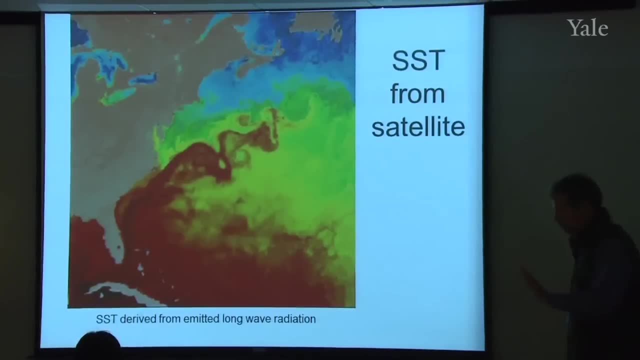 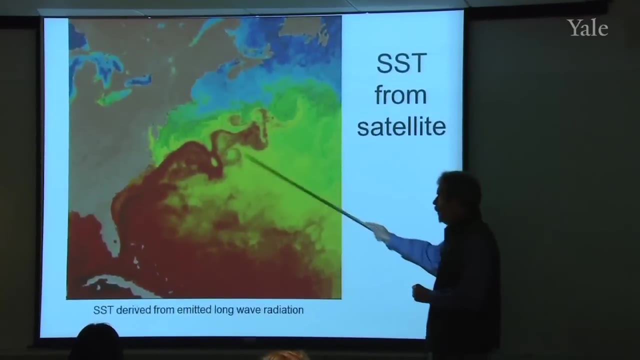 He doesn't show anything splitting off to go up north the way the previous diagram did. Here's a satellite image. One really neat way to look at this is just to take an infrared, a thermal infrared image of the ocean, play some tricks to get rid of the clouds and then interpret the 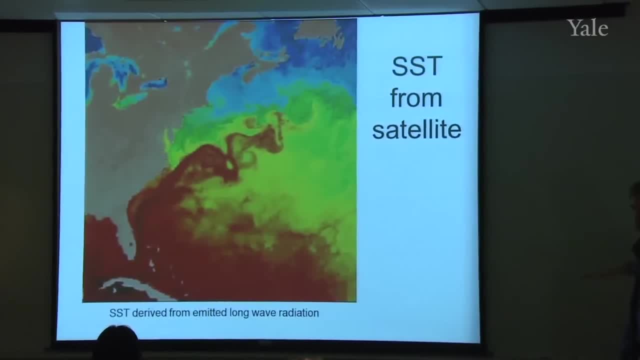 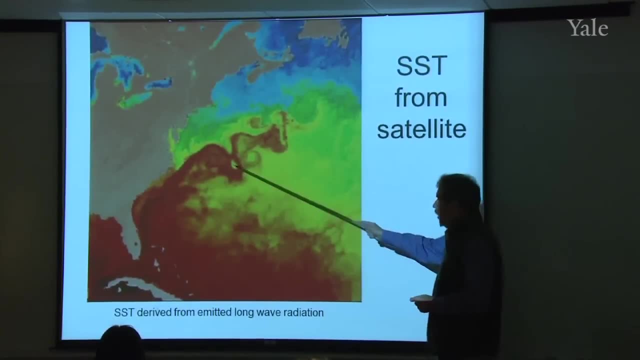 intensity of that radiation as the temperature of the emitting object. Remember the Stefan Boltzmann law: The warmer an object is, the more it radiates. So that's what's done here. A color code has been applied. The red is areas that are emitting strongly in the 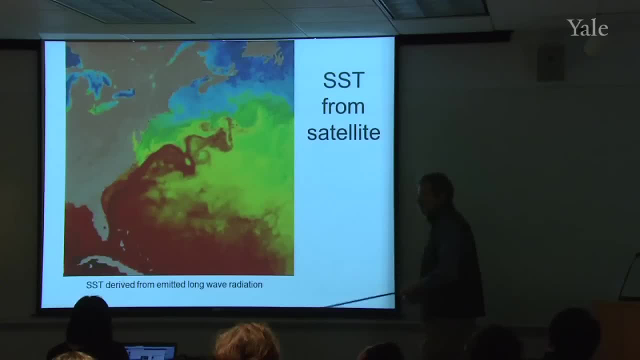 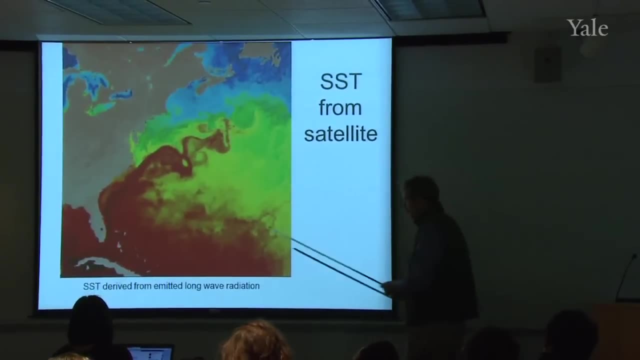 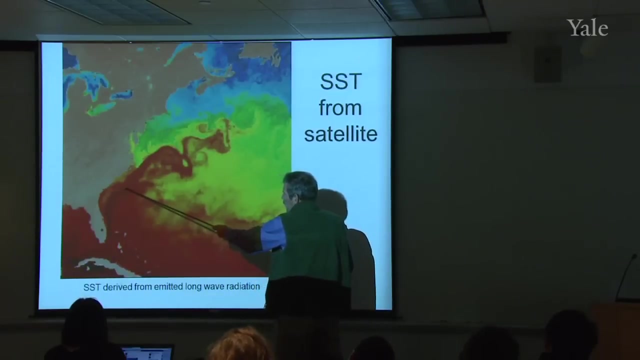 thermal infrared. The blue are areas that are emitting less strongly, And then that's directly related to the temperature of the sea surface. So this is sea surface temperature, Warm water in the tropics And then this little stream of very warm water coming up here. 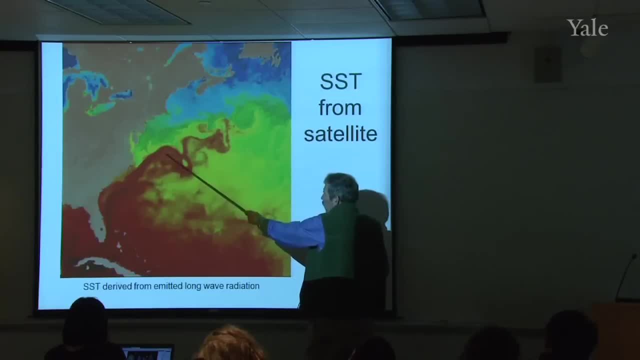 It's getting mixed in a little bit, but it continues as a warm water current until it leaves Cape Hatteras. We see it continuing, but as soon as it leaves it begins to meander and you form eddies on both sides, cold eddies on the. 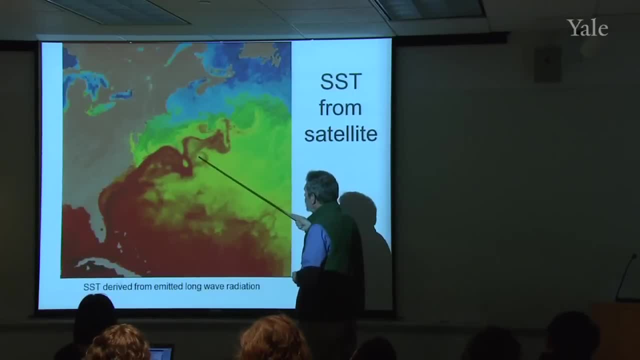 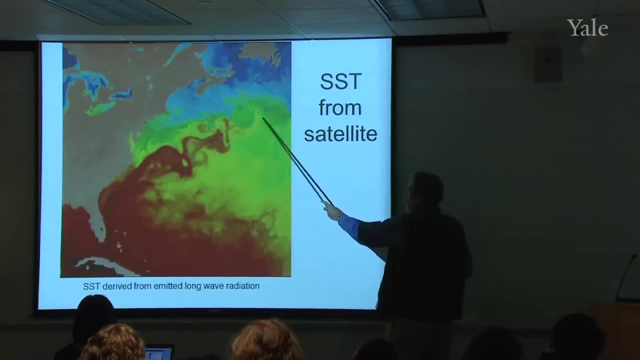 south, warm eddies poking through from west to east, warm eddies from east to west, and it begins to mix in. However, you can still see remnants of it further across the ocean and it still has a pretty good speed there. but 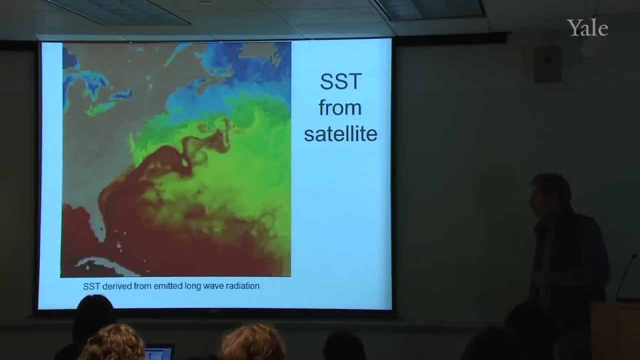 it's losing some of its thermal characteristic as it mixes in with the environment. So that's a good view, But remember, this is going to be changing with time, So if you were to take another image a week or so later, it's. 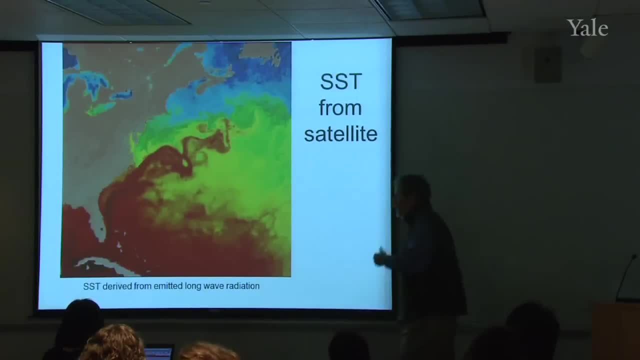 If you took it just a day or so later, it would look a lot like this. But if you waited a week and took another image of it, those eddies would have moved around quite a bit and new ones would have formed and it would look quite different. 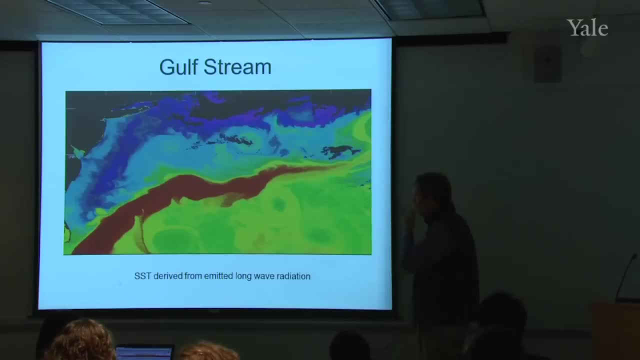 Here's a zoom in on another date. Again, the trick is the same. We're looking at sea surface temperature derived from emitted longwave radiation, And here's Delaware Bay, Long Island Sound and there's just a little bit of the tip of Cape Hatteras. 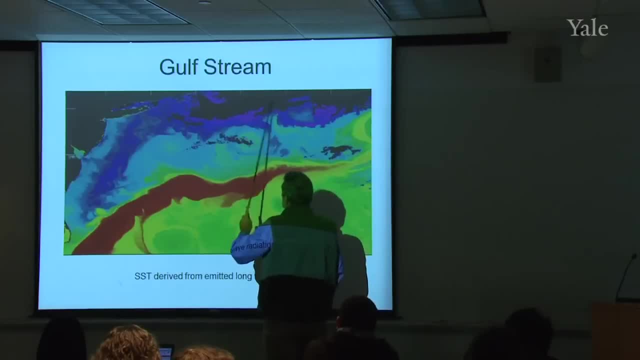 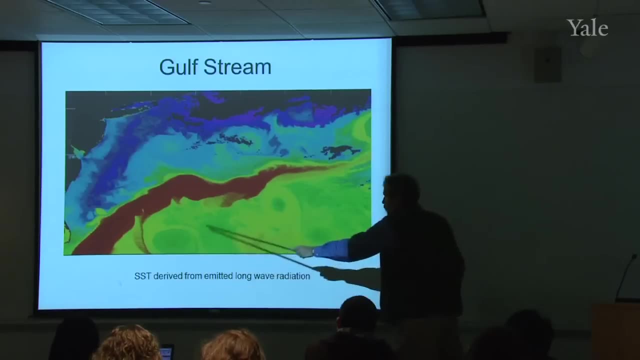 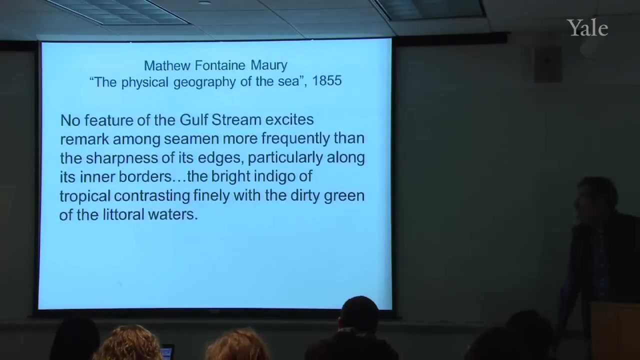 So you see the warm water coming up here- This may be a little bit of the Labrador Current coming down in here- And then you've got the mid-ocean, the Sargasso Sea, out here in the middle. A quote from one of the first books to lay down a. 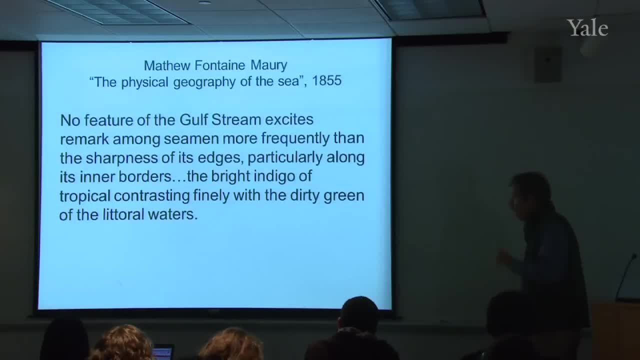 description of this was a book by Matthew Fontenot. It's called Montaigne Mori in 1855, where he was working for the Navy and he gathered together information from ship's logs from all the US Navy ships and wrote this: 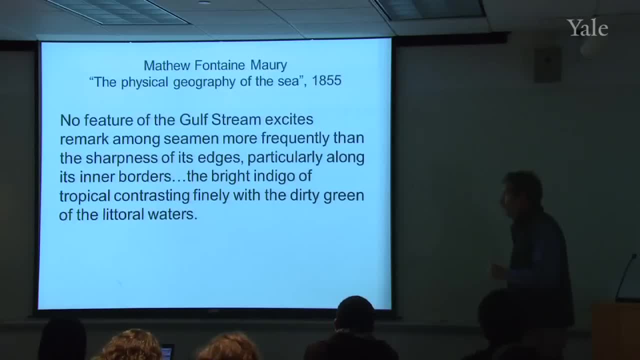 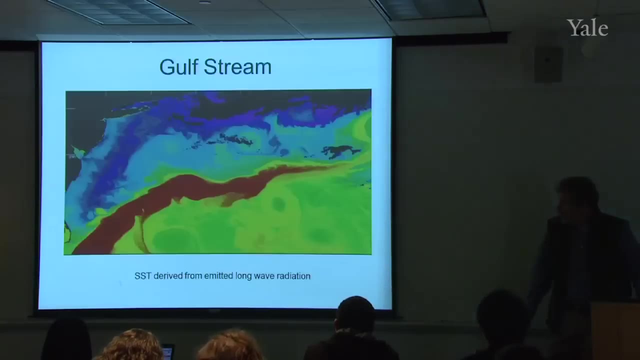 rather remarkable book called The Physical Geography of the Sea, And here's a quote from that book. No feature of the Gulf Stream excites or marks among seamen more frequently than the sharpness of its edges, particularly along its inner borders. He's referring to this edge here. 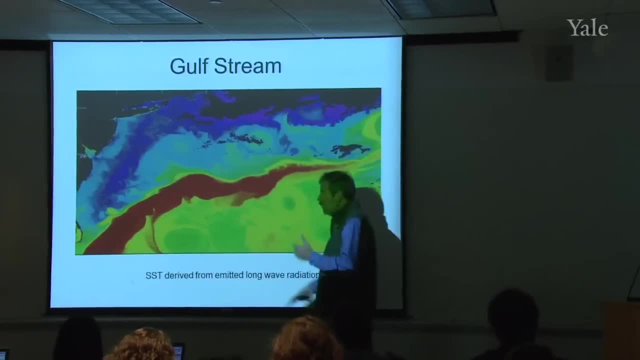 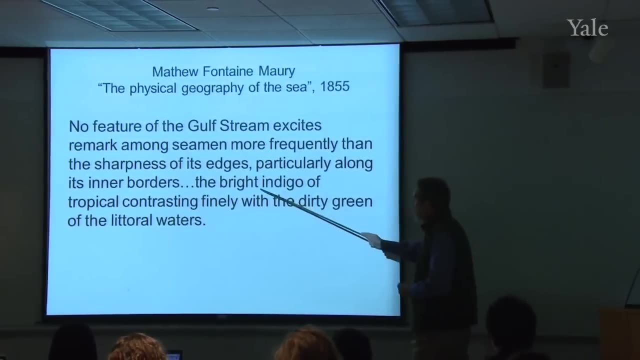 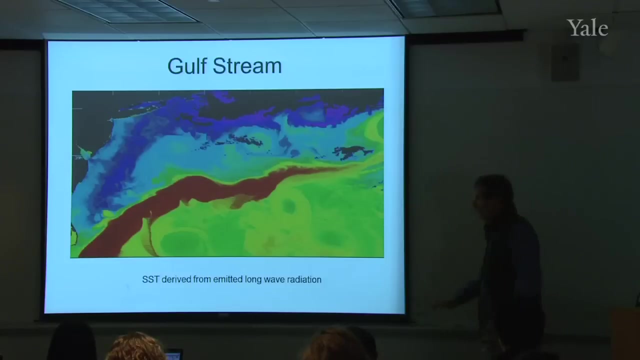 When you sail across that, you really notice that boundary, in part because of what he says. The color of the water changes from the bright indigo of the tropical to the dirty green of the literal. So you're getting this. water is basically a clear tropical. 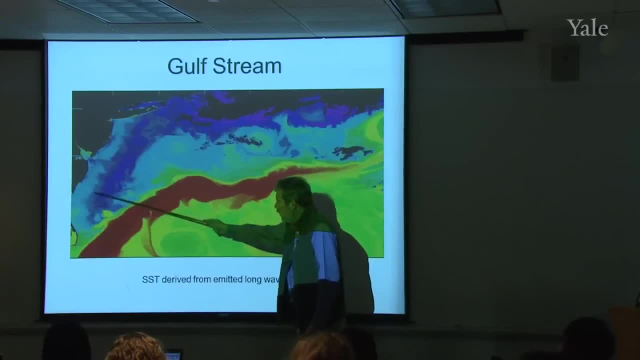 light blue, but the water back here is rather dirty and green, And you see that boundary very, very sharply as you sail across it. There are other things that you can see. There are other things, though, that a sailor would notice as well. There tends to be cumulus clouds, often over the warm Gulf Stream but not over the cold water. That's to be expected, because the warm water would destabilize the atmospheric boundary layer and cause thermal convection. So when you're approaching that, you can often see it at. 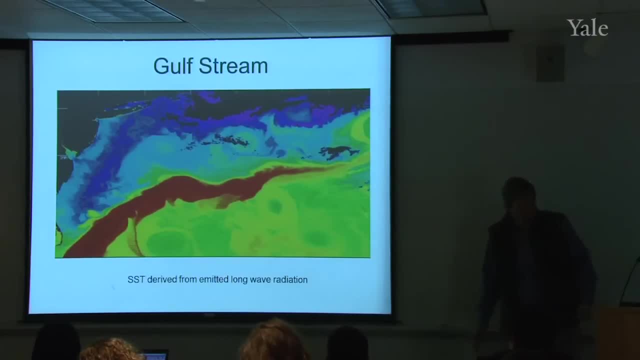 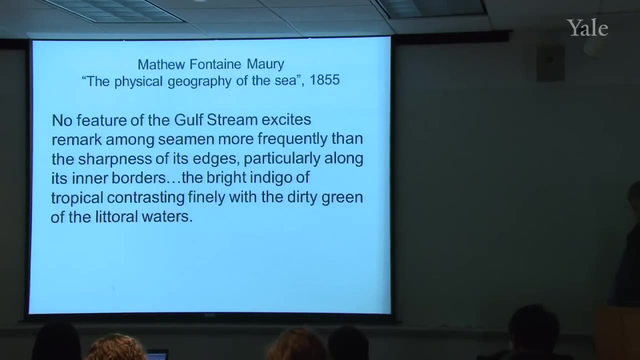 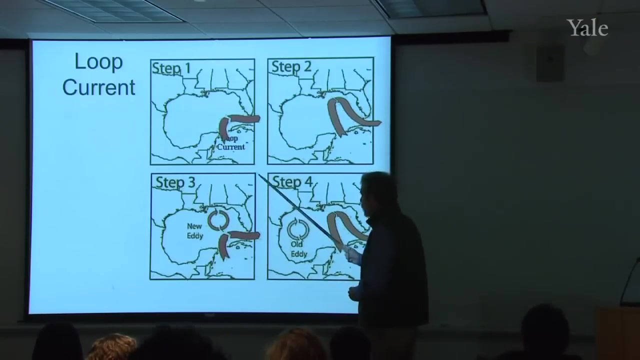 quite some distance, because you see cumulus clouds are building up over the Gulf Stream. Questions. Now, what about this Gulf of Mexico thing That's rather interesting? It's called the loop current, Remember, as part of the North Atlantic Gyre. you've got water. 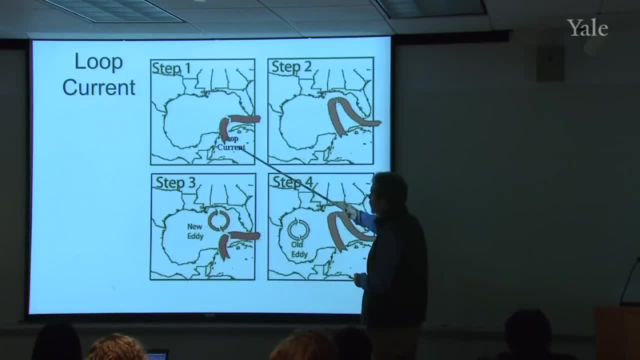 pushing in to the Caribbean Sea, then coming up into the Gulf of Mexico in a well-defined current. But that current is not steady. It changes from week to week and it goes through a cycle of a rather interesting cycle. For a few weeks it'll seem to turn directly eastward and end. 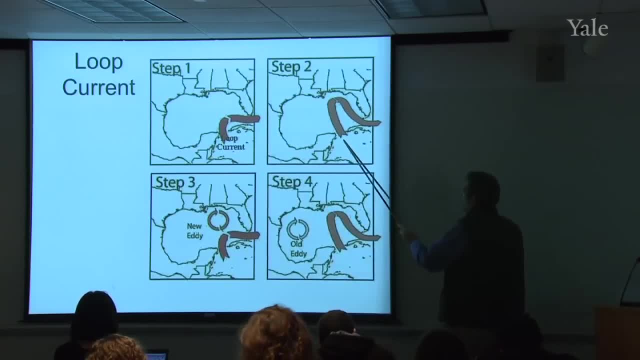 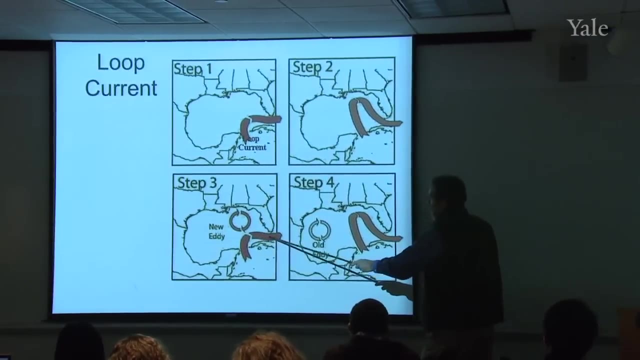 up in the Florida Current. Then that loop seems to elongate. Then that will break off. It'll form a clockwise eddy which will then drift off, and the shortcut is then re-established. It's more like this: That eddy will eventually drift into the western part of. 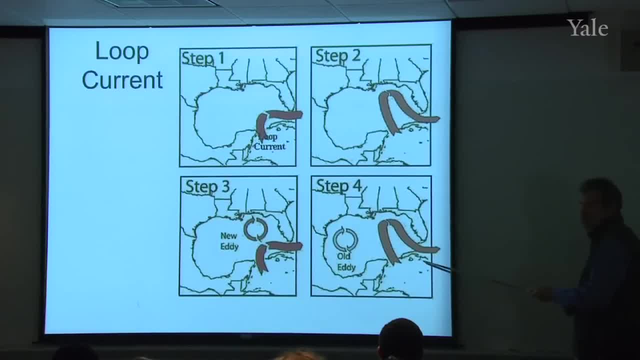 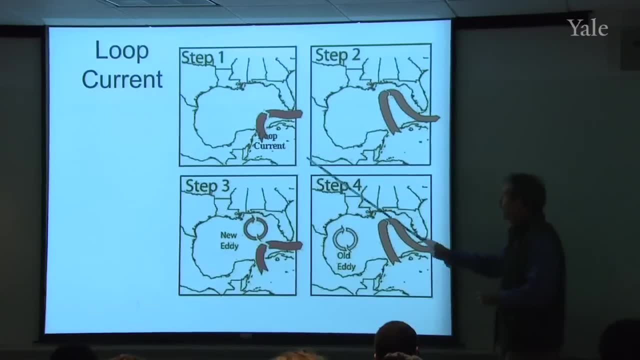 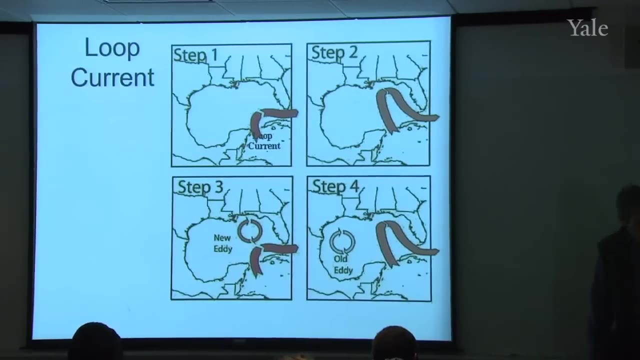 the Gulf of Mexico, And the cycle will then continue. So it's an unsteady current going through, this cyclic behavior of taking a shortcut, extending in a long path and then breaking off into a new eddy, And you can see that in satellite images. 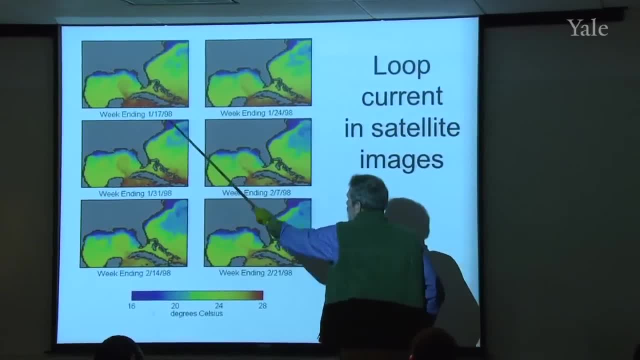 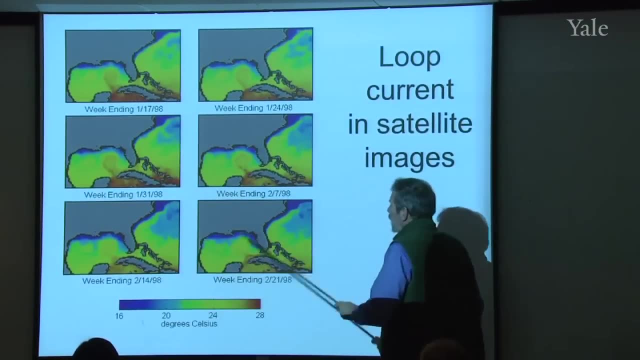 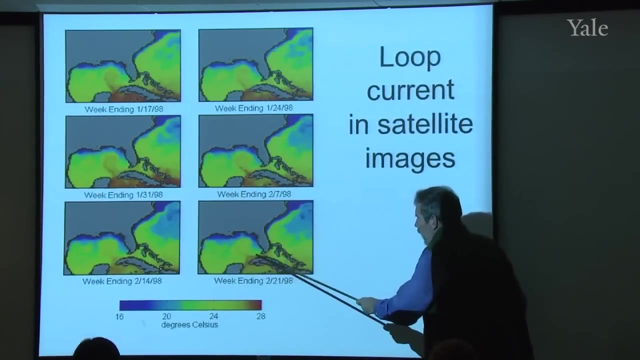 And here's a sequence of satellite images And the dates are given here. They're from 1998.. But there's the loop, And then as it drifts, And then as it goes westward and weakens, the new direct link is established there to get the water into the. 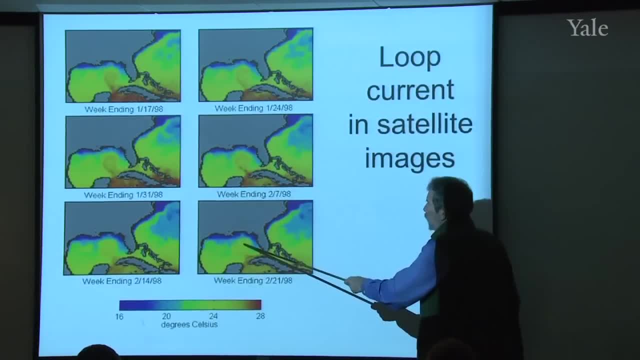 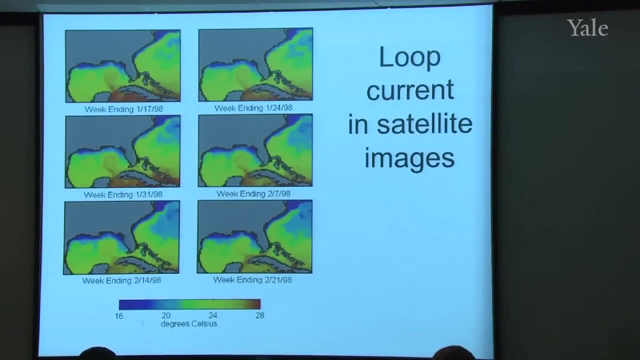 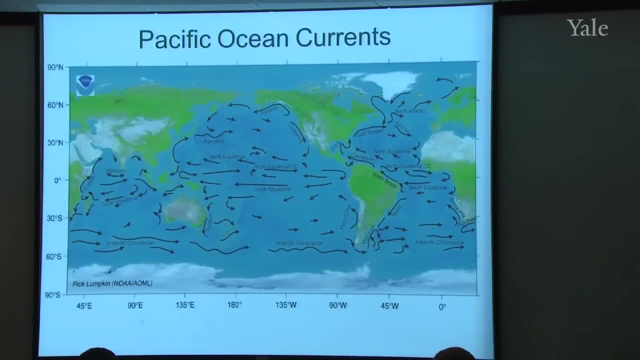 Florida Current. So, depending when you're down there, you're going to find either a lot of warm water here or not, depending where you are in the phase of this cyclic alteration. OK Well, I'm not going to go into the Pacific Ocean Currents nearly. 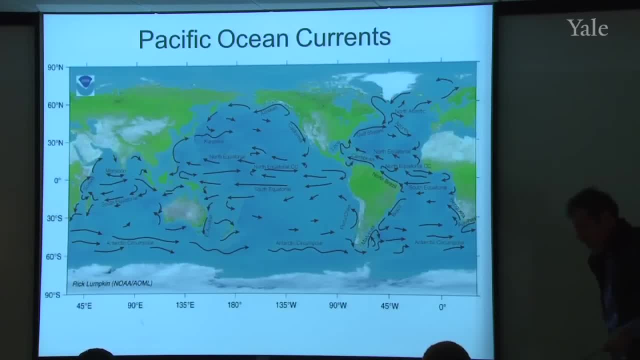 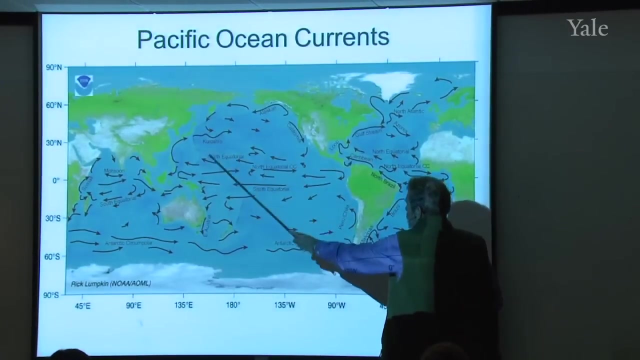 OK, as deeply. If you want to take a course in this, you can take a course in physical oceanography and learn about each of these ocean basins in a more complete way. But I will say that there are certain parallels. You've got a North Pacific Gyre, just like you had a. 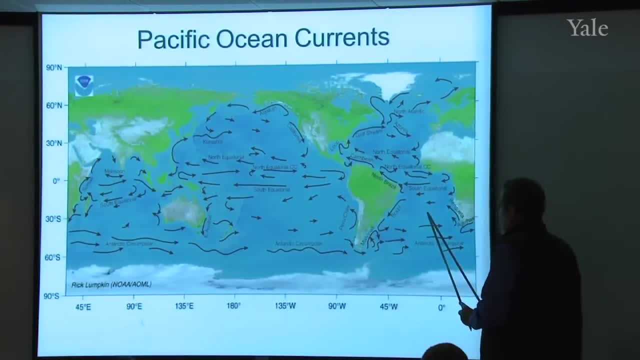 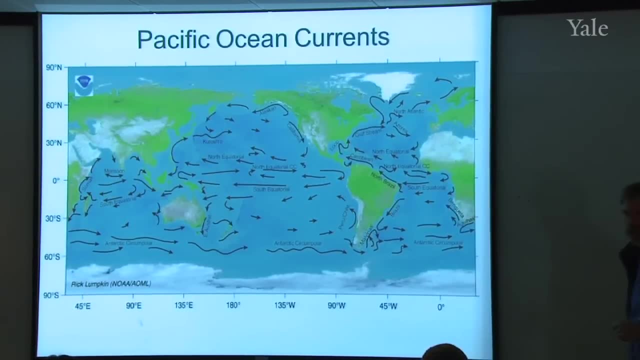 North Atlantic Gyre, A South Pacific Gyre, just as you had a South Atlantic Gyre Here. the current is the Peru Current, sometimes called the Humboldt Current, And then the South Equatorial Current, the East Australian Current, and then it returns here. 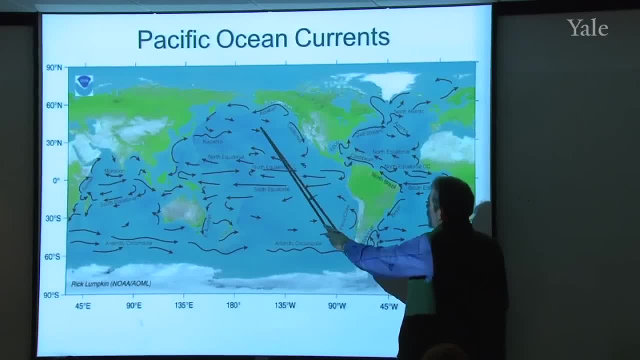 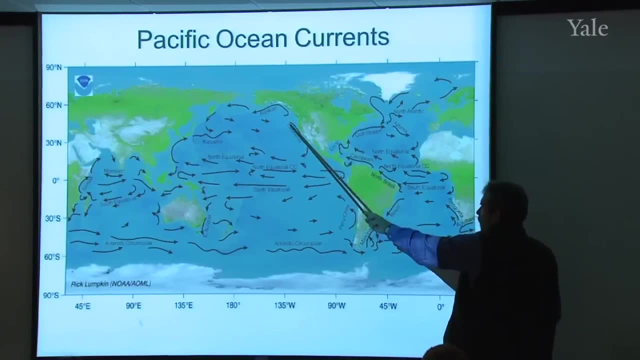 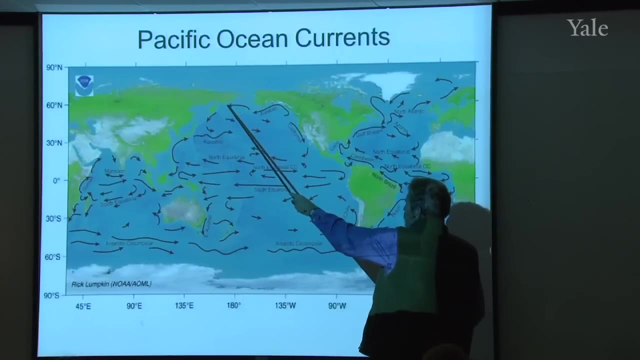 The one surprise perhaps is this Alaska Current, So you get the current coming across here from the Corotio. that then splits. Some of it comes down the California coast and some of it returns in the other direction back across the northern stretches of the Pacific and returns into the. 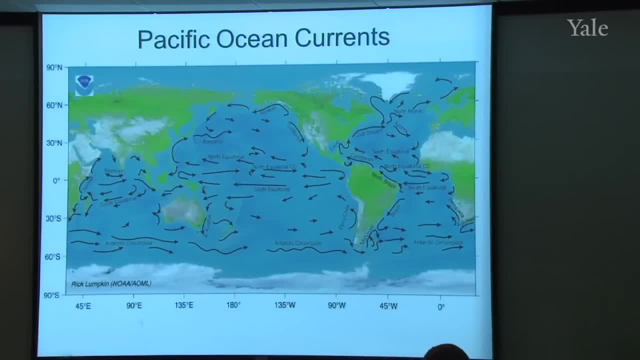 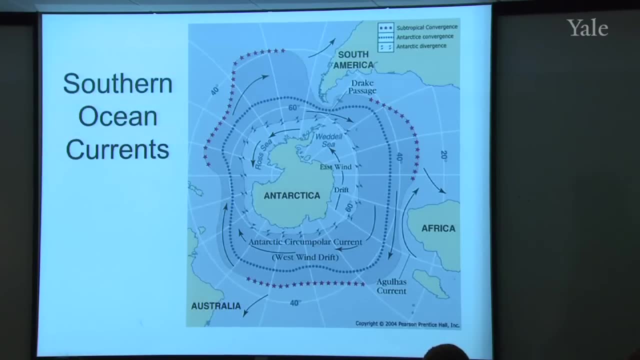 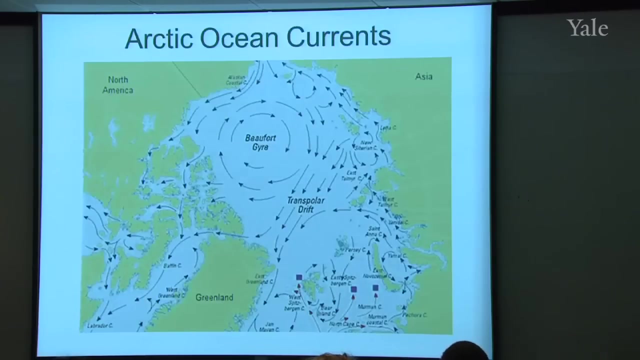 Corotio. that way, The Southern Ocean has its own current system. That's the Antarctic Circumpolar Current, sometimes called the West Wind Drift. It pretty much goes all the way around Antarctica And in the Arctic Ocean you've got a well-defined 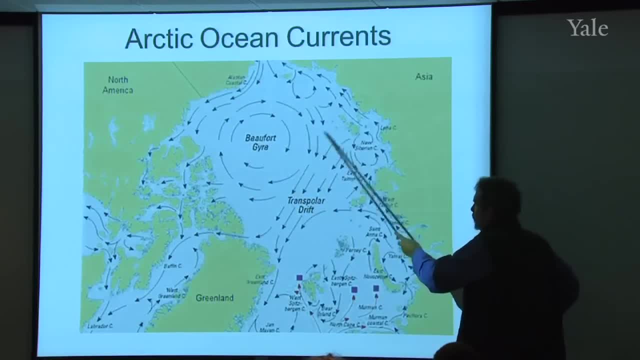 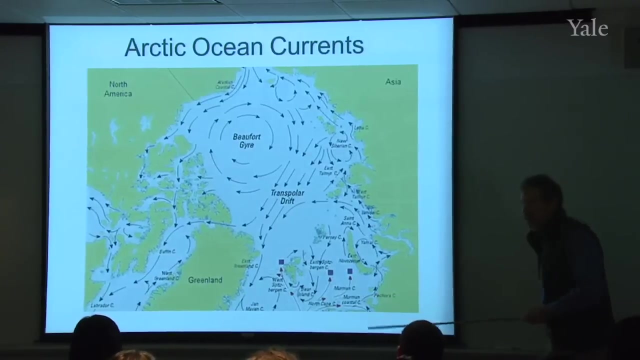 gyre called the Beaufort Gyre, And then, as part of that or consistent with that, is a current that runs kind of across the basin from one side or the other, called the Transpolar Drift. Now there is water leaking in and leaking out of the Arctic. 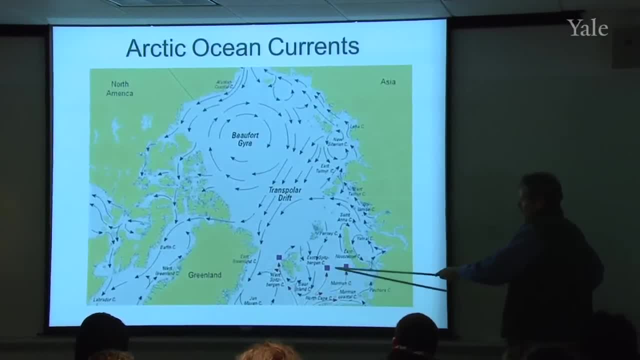 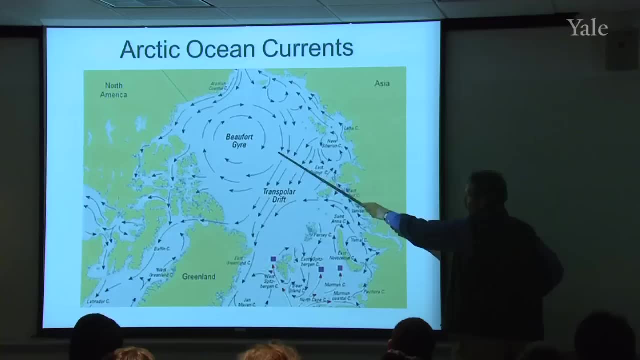 Ocean. I've already mentioned that the Gulf Stream extension will come up here and water then will enter the Arctic Ocean, stay there for several years presumably, and then some of it will leak out And the East Greenland Current will come out that way. 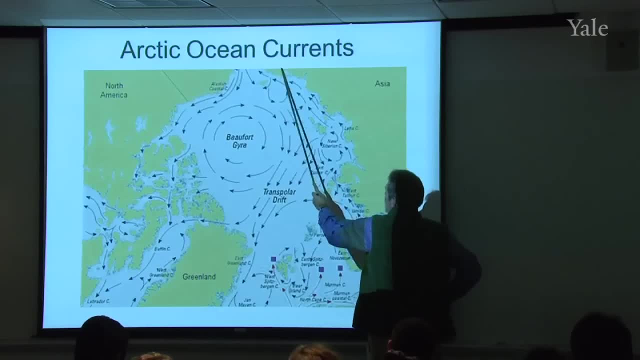 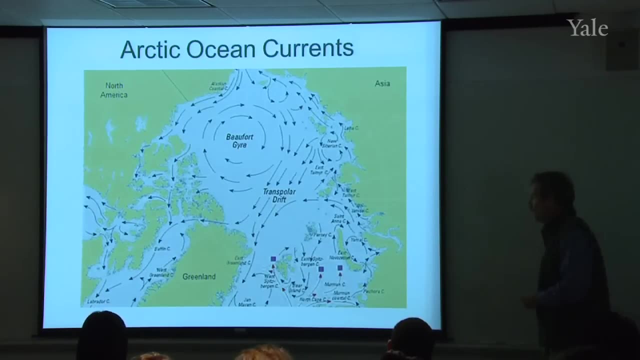 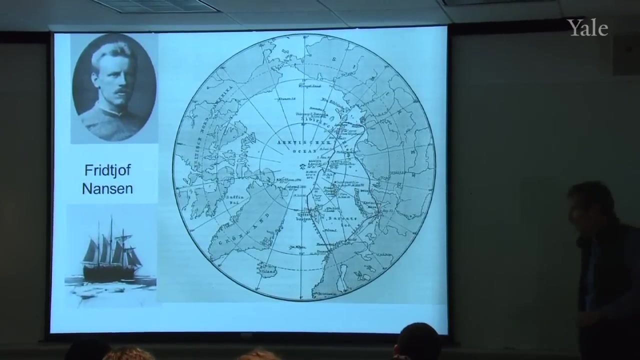 There's also some exchange between Alaska and the Soviet Union. There's some exchange of water there as well, between the Pacific Ocean and the Arctic Ocean. One of the interesting stories about this Transpolar Drift is the trick that Fritjof Nansen tried. 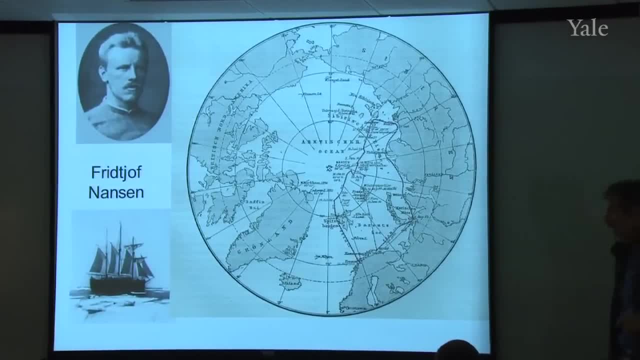 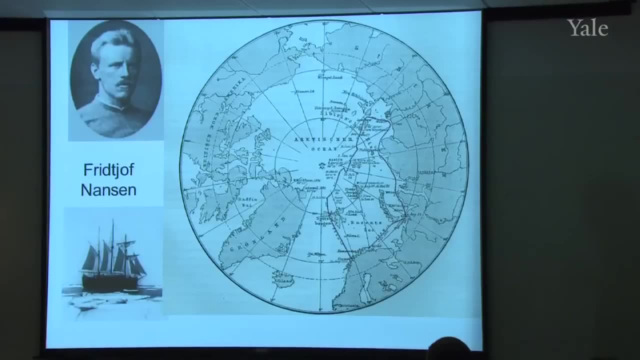 Now, you already know that name because he invented the Nansen bottle. but this was really his claim to fame. He wanted to be the first one to run, He wanted to be the first one to reach the North Pole. And he figured: why should he have to work at it? 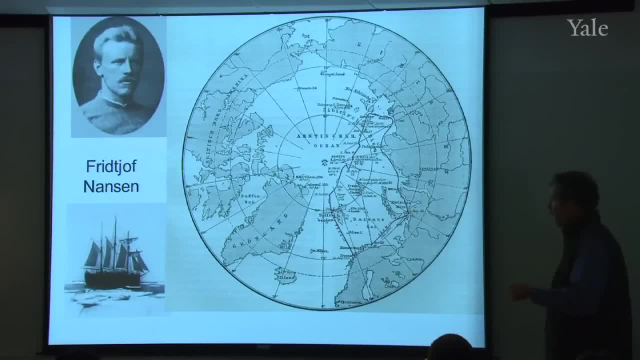 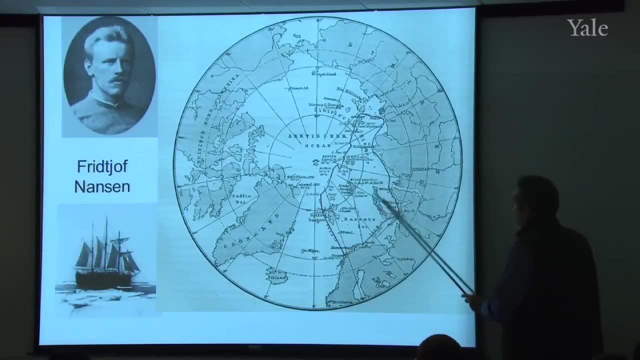 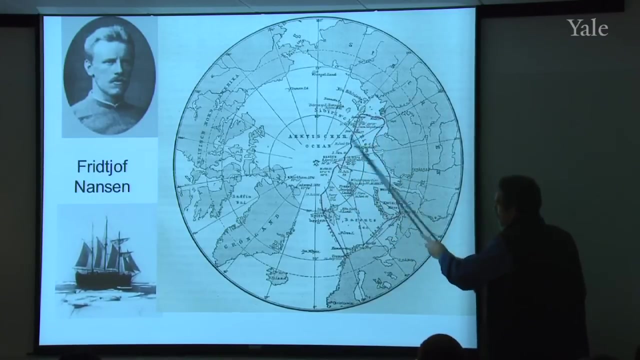 Why shouldn't he let nature do the work for him? He already had some evidence that the Transpolar Current existed. So he said, if I can just get my ship locked into the ice about here, it should carry me close to the North Pole. 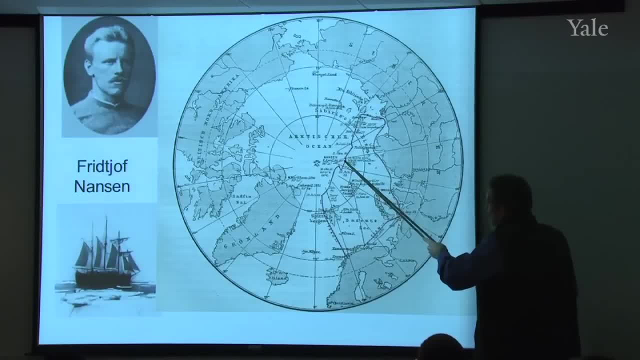 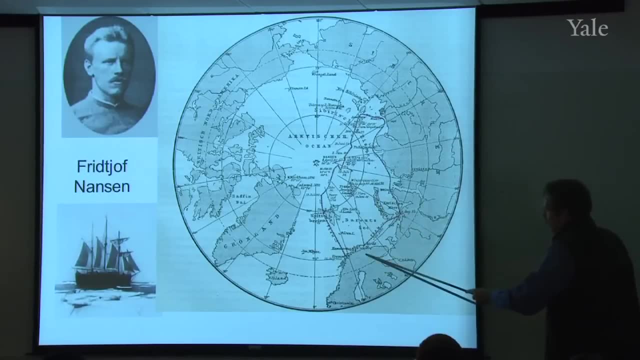 And he did that. He left the ship here and tried to do the rest of it by land- not by land, but over the ice. couldn't make it and ended up having to travel on the ice all the way back to here, where he finally got back to. 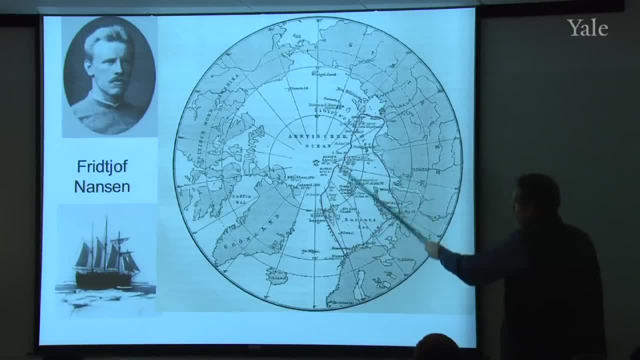 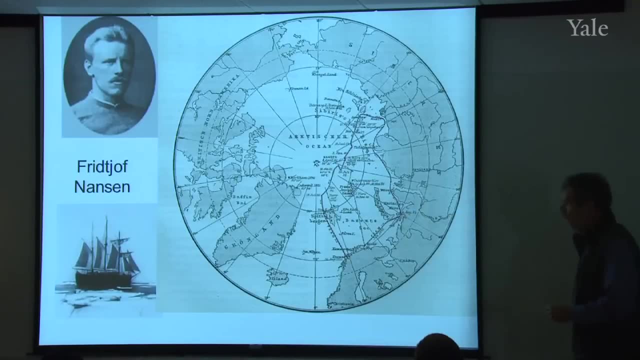 civilization while the ship continued to move like this. So it was a good idea, but it didn't quite get him close enough to allow him to reach the North Pole in that way. But it's a great adventure book If you want to read about one of the great adventure stories. 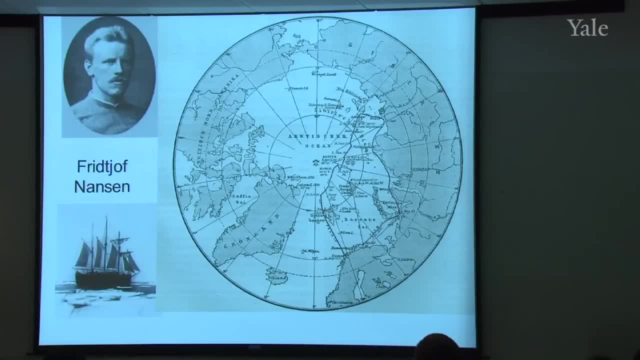 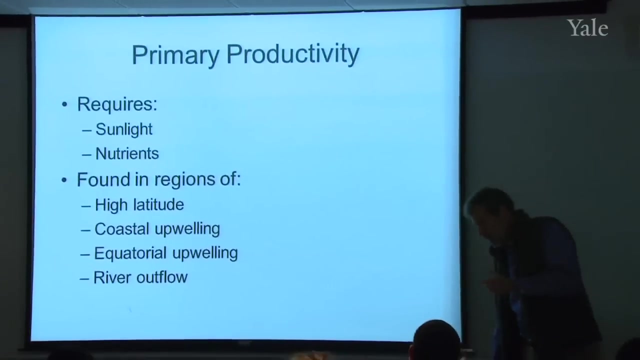 in human history. read about Nansen's attempt to get to the North Pole using that Transpolar Drift Questions here. OK, Switching gears slightly. we're interested in the relationship between physical oceanography that we've been talking about so far and biological oceanography. 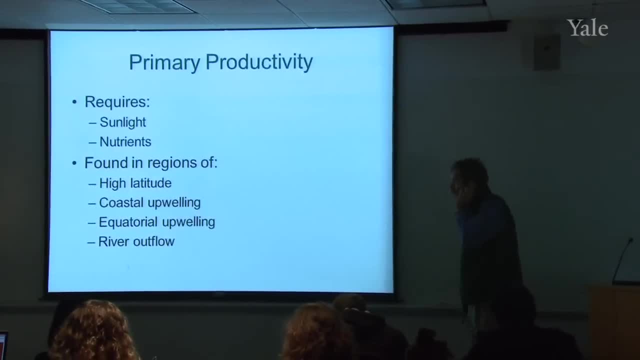 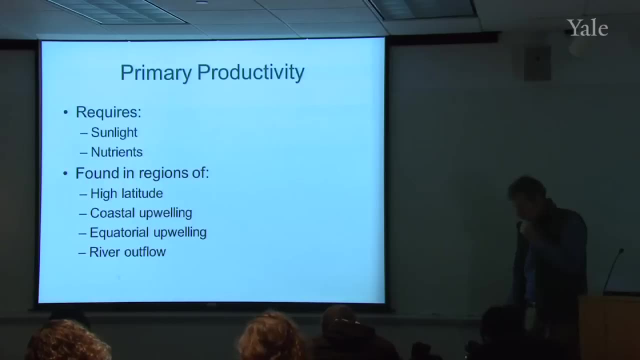 In particular, what is it that controls productivity in the world ocean? By this I mean biological productivity, Now the way a biologist approaches the question is: what is it The way a biologist approaches? this is first to understand the food chain. What feeds on what? 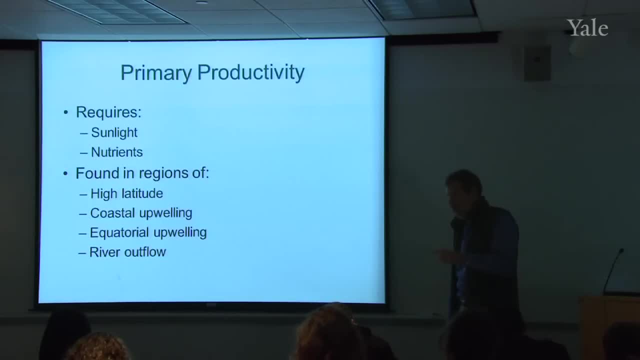 And I'll show you that in just a minute. But the most basic level, where the food chain begins, is called primary productivity, And it's usually referring to plant life in the ocean. Plant life requires sunlight and nutrients. You need to get those two things together in order to get 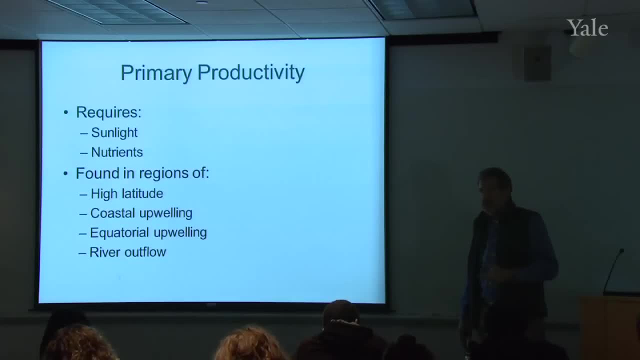 the primary productivity- OK, Primary productivity, And then the rest of the food chain builds on that And, as I'll be showing you, there are vast parts of the ocean that are devoid of any primary productivity And, for that reason, largely devoid of any biological. 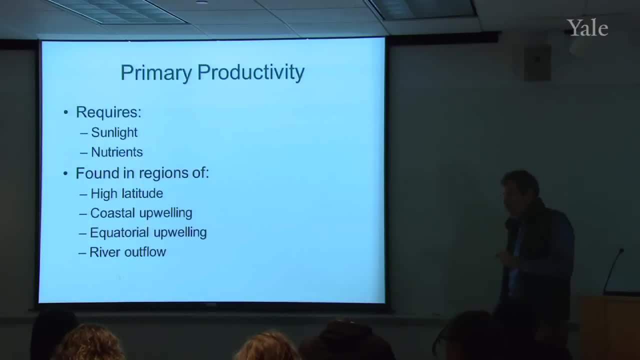 activity at all. But there are other regions in which biological activity is very, very active And if I had to categorize them- and I'm going to try to categorize them- I would put them into those four categories. There's a lot of primary productivity in high 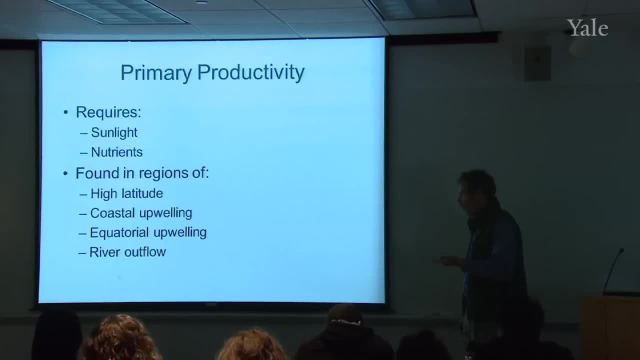 latitudes in regions of coastal upwelling, in regions of equatorial upwelling and in regions of river outflow, And, for the most part, the rest of the ocean is very limited, if not completely devoid of primary productivity. 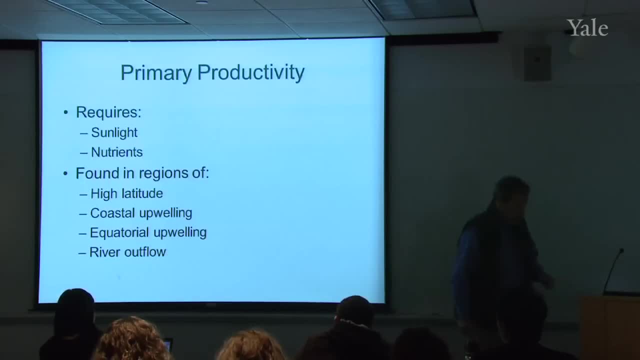 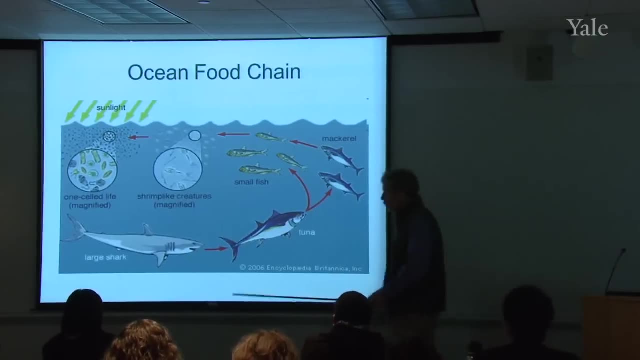 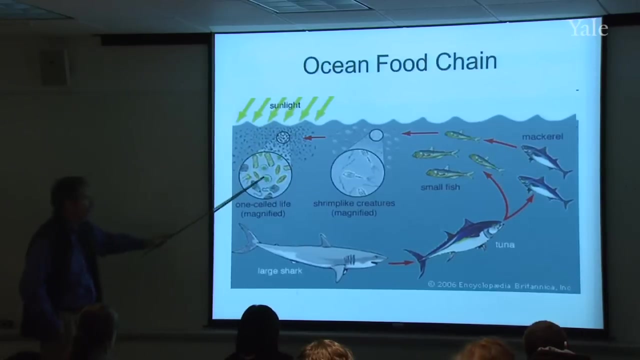 So in the next few minutes we're going to talk about this kind of way of understanding productivity In the oceans. So here's a typical food chain. You start with single cell life. that are plants, And they require sunlight and nutrients especially. 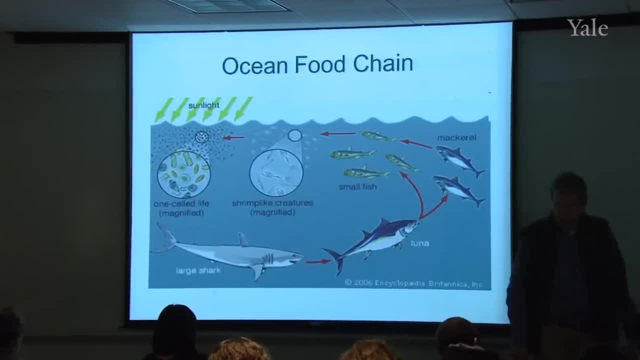 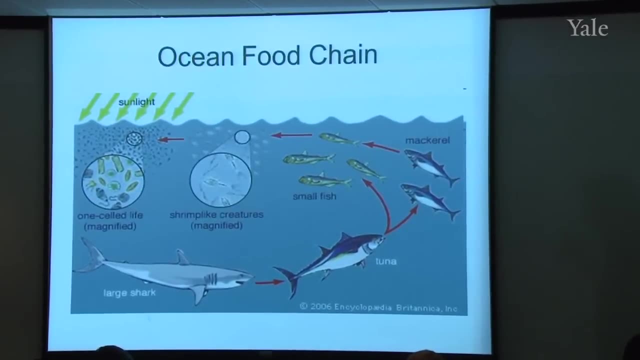 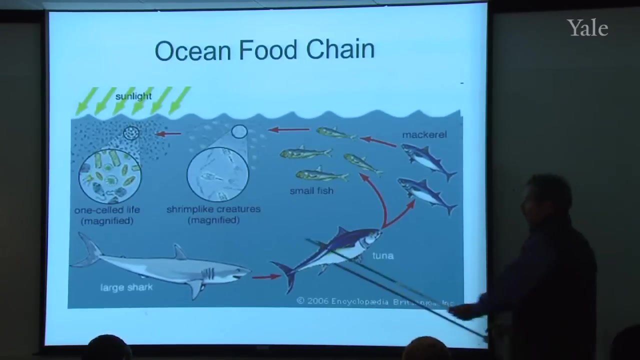 phosphorus and nitrogen. It's a carbon-based life, but there's plenty of carbon available, So it usually depends on the phosphorus and the nitrogen that allows that to get started. These organisms get eaten by small animals, so-called zooplankton. 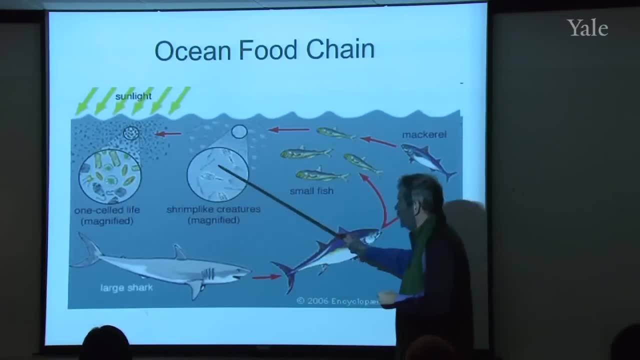 These are so-called phytoplankton. They get eaten by zooplankton And then in turn eaten by small fish, larger fish, larger fish and so on. So that's the base of the food chain. That's the primary productivity there. 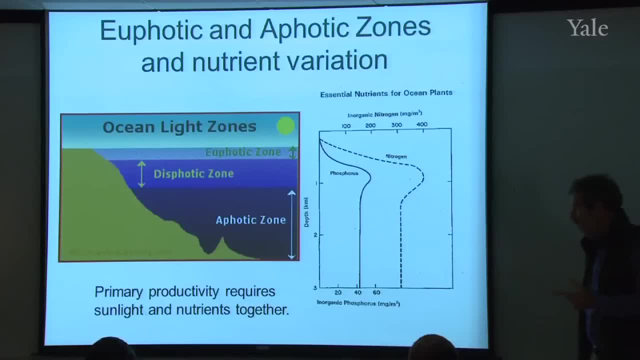 Now here's the great difference, Here's the catch-22 for ocean productivity. You need light from the sun, but light is absorbed rather quickly as you go down into the ocean. The region that has lots of light in the ocean, the upper. 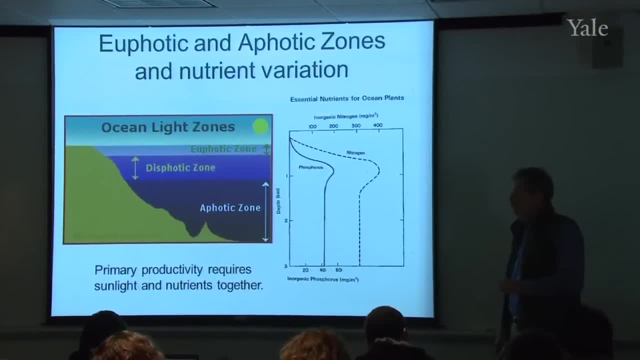 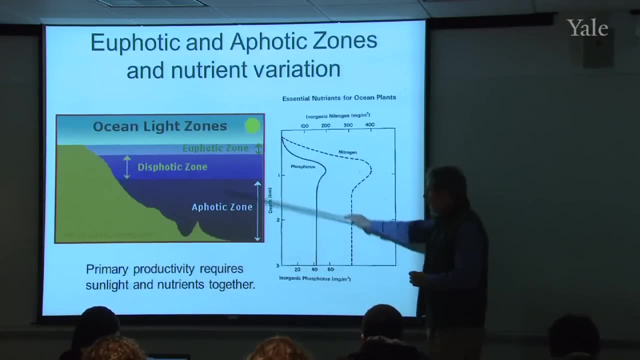 50 or 100 meters is referred to as the euphotic zone, E-U-P-H-O-T-I-C, The euphotic zone. There's a layer beneath that that gets a little bit of light, And then, however, most of the value of the food chain is the 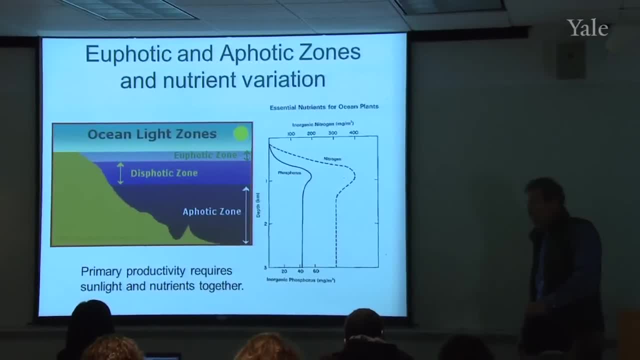 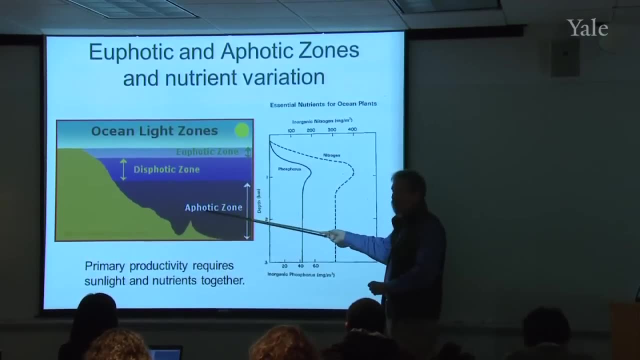 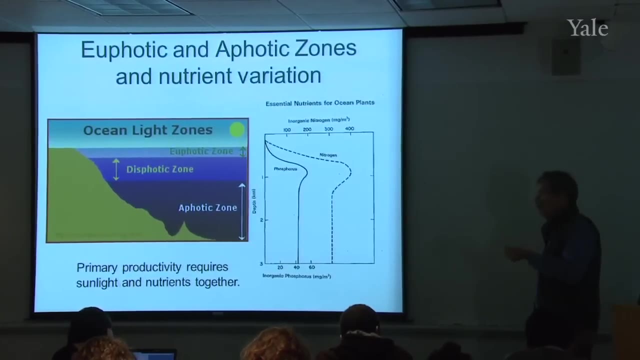 vast majority of the ocean depth is dark because the sunlight doesn't penetrate that far. That's the aphotic zone. Aphotic meaning no light. On the other hand, if you look at the concentration of nutrients in the ocean- and here it's plotted versus depth, 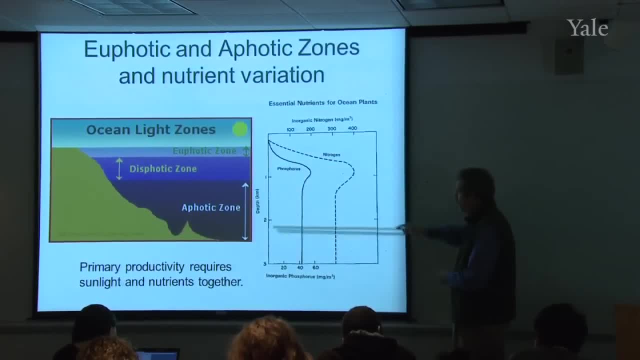 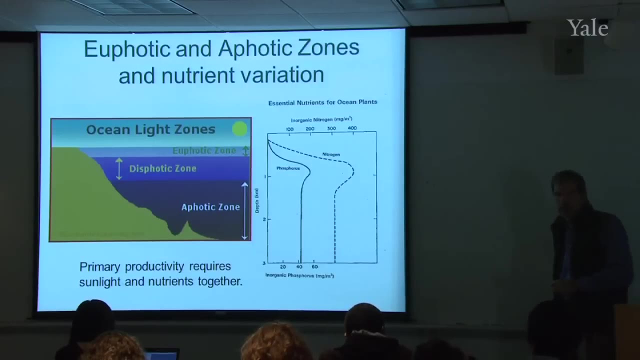 in kilometers sea surface, one kilometer, two kilometers. Most of the nutrients- phosphorus and nitrogen- are in the lower parts of the ocean And in the upper parts of the ocean, where you have the light, you have depleted nutrients. 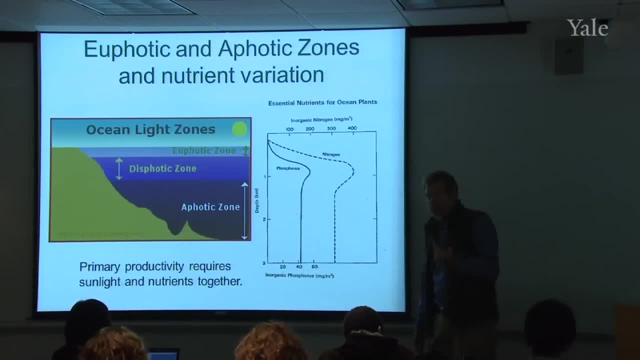 So here's that catch-22.. Where you've got light, you don't have the nutrients. Where you've got nutrients, you don't have the light. That's the great break upon ocean productivity. To get ocean productivity, you've got to violate this. 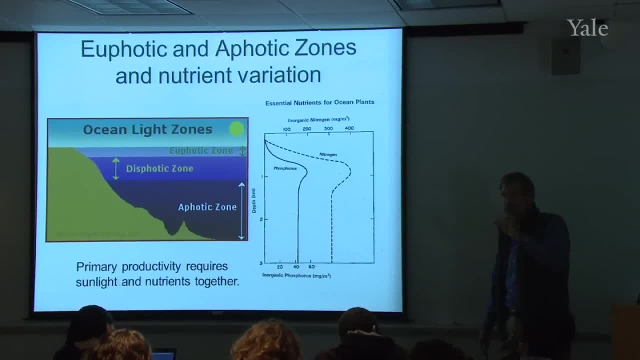 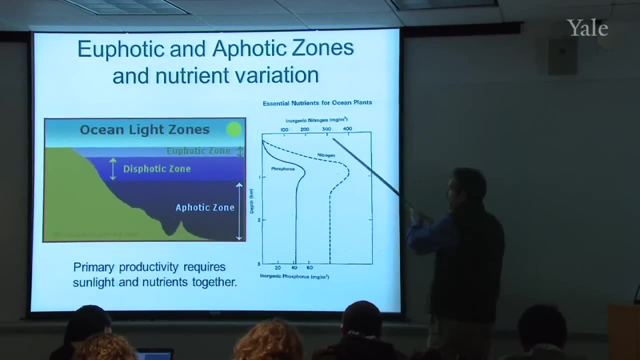 general anti-correlation and get the two together. You can't get the sunlight deeper, So the only way to do that is to get some of these nutrients up to the surface, And that'll be the focus of our discussion for primary productivity. How can we get some of these nutrients up to the surface? 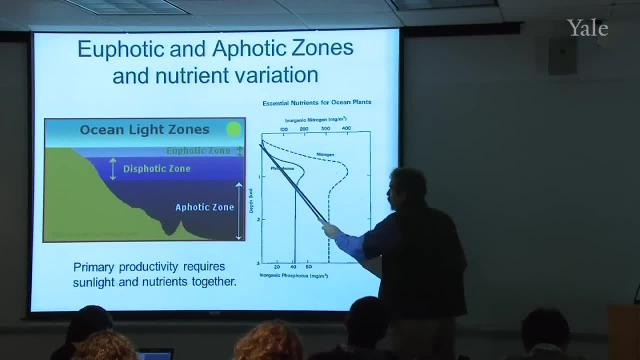 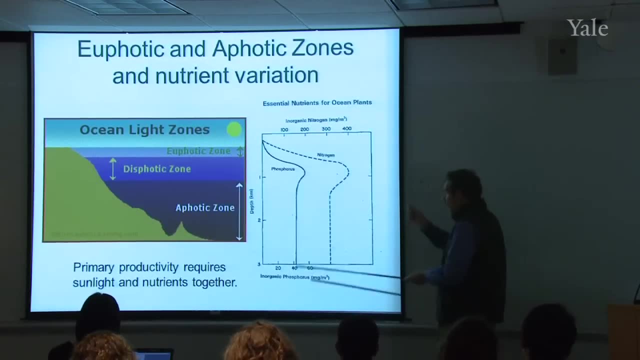 Now, why is it like this? Well, it's because you've had some blooms of phytoplankton. They've depleted the nutrients And then their bodies will fall gravitationally into the lower ocean and then rot And the nutrients are released. 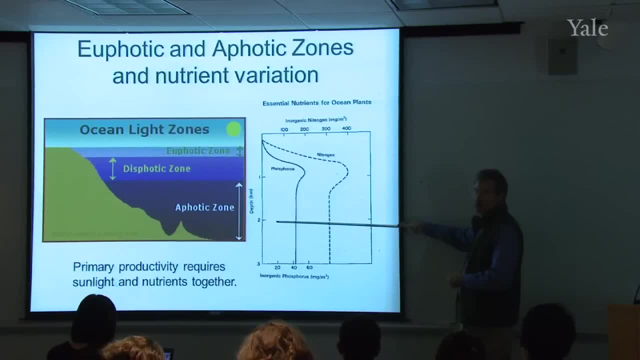 The nutrients are released again, but because of gravity they're released in the lower parts of the ocean, And once that has happened, then you have that depletion And at least in this simple set of plots, the productivity would shut down. You need to do something to re-establish concentrations of 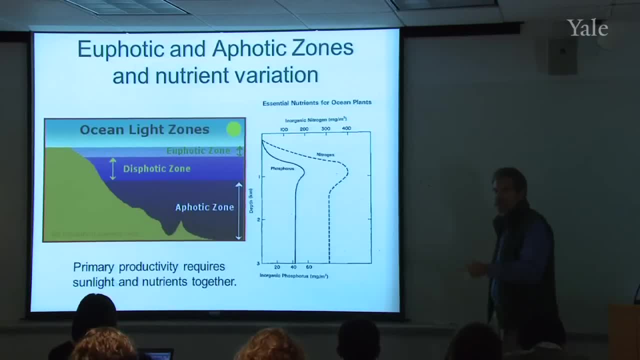 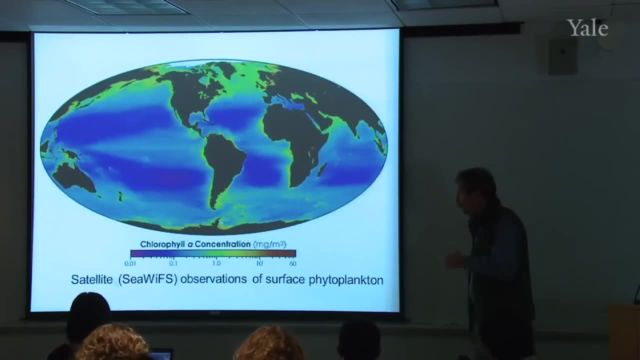 nutrients in the surface waters of the ocean in order to get the primary productivity re-established. This is one of my favorite diagrams. It comes from. It's a satellite in orbit called SeaWiFS, which looks down at the surface of the ocean and, by using two 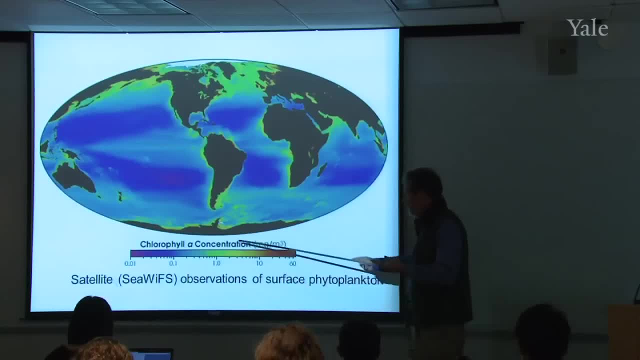 channels, two reflected channels. it maps out the concentration of chlorophyll- chlorophyll A in this case- in the surface waters of the ocean. So in a way it's detecting those phytoplankton directly, because they have chlorophyll in their bodies. 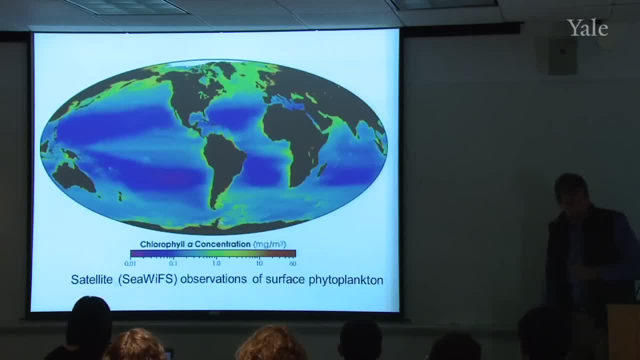 And so here we have a global map of the primary productivity in the ocean. It's a remarkable map. It's a remarkable thing. And the scale here, it's a log scale. The units are milligrams of chlorophyll per cubic meter of. 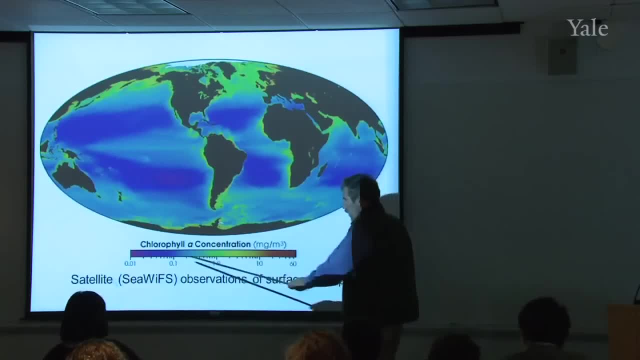 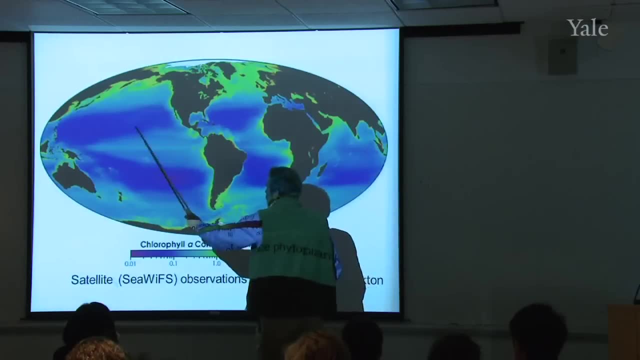 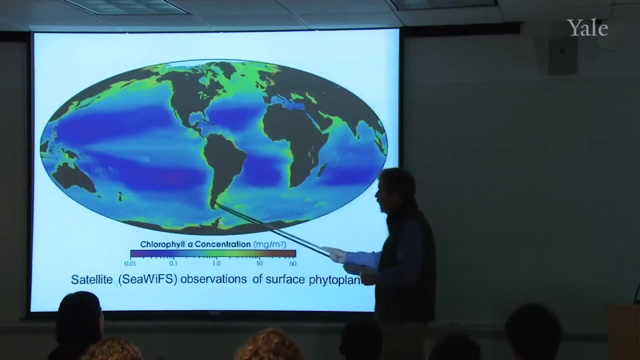 ocean water going from 60 units on down to 0.01 on a log scale. So the purple areas are biological deserts. There's really very little primary productivity going on in these areas. We can imagine why that is, because- remember that warm. 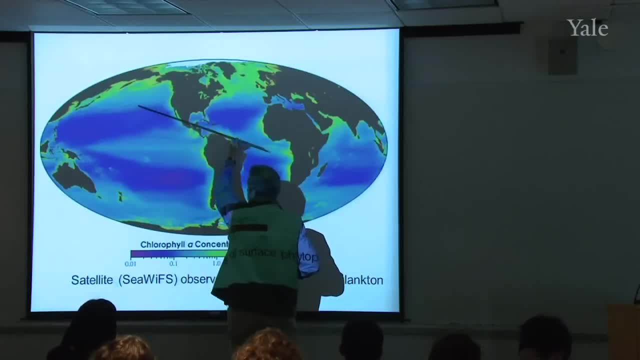 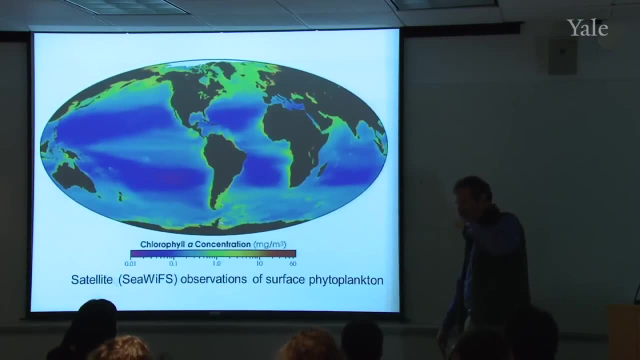 water lens extends from there There to there, And so you've got this layer of warm water floating on the sea, very strong thermocline beneath it which, just like an inversion in the atmosphere, makes it very difficult to mix water vertically. 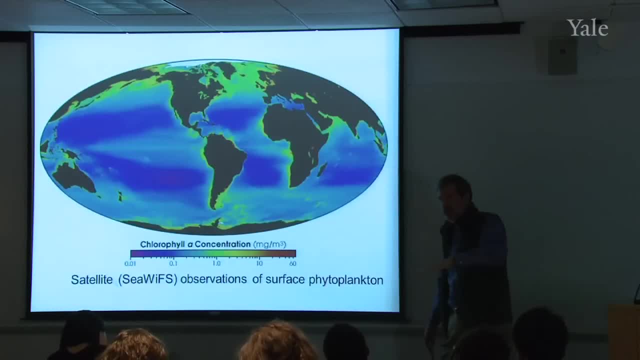 So while you probably have a lot of nutrients just a few hundred meters down, because of that static stability in the thermocline you can't mix it to the surface. So let's talk about the high latitudes. I'll go through and check off the four items I had there. 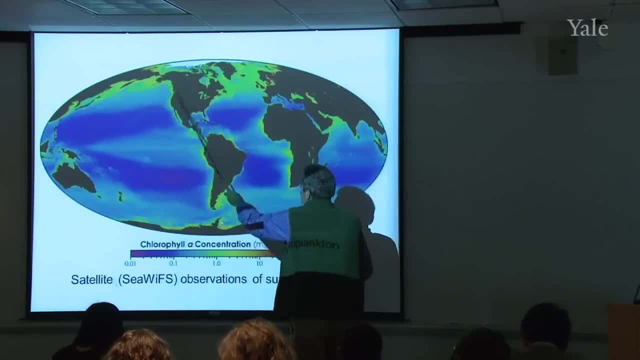 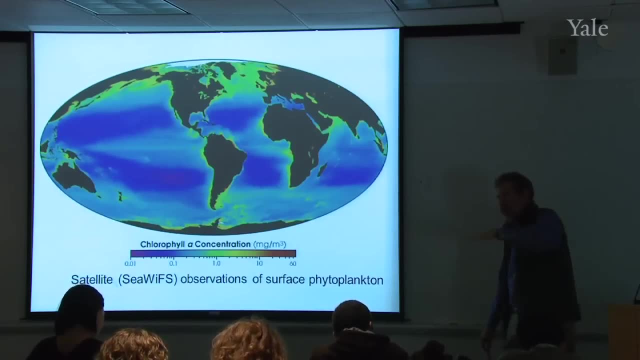 High latitudes are generally high productivity. Well, that's because that warm water lens doesn't extend to high latitudes. You've got cold water at the surface, You've got cold water at depth. You don't have a strong thermocline in the. 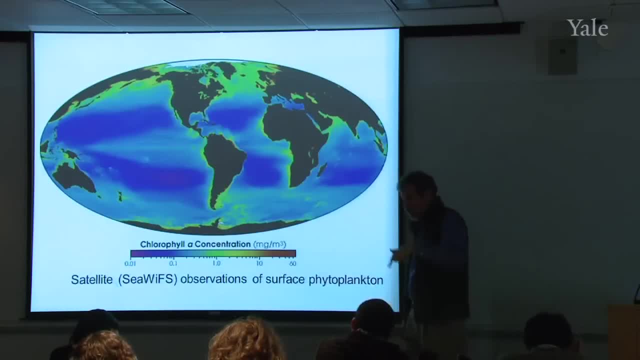 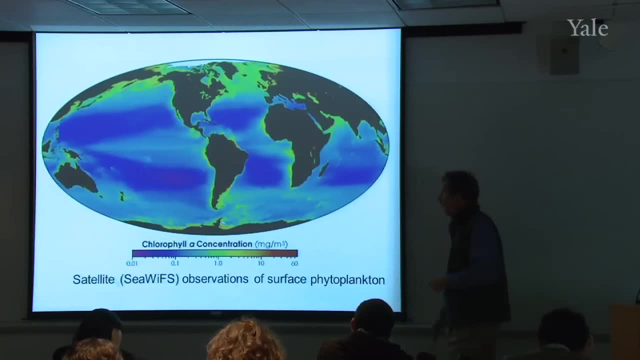 high latitudes. You do have also strong storms in the atmosphere, putting winds on the surface of the ocean, tending to mix things, So it's pretty easy to get water to mix up and down when you're in the high latitudes. 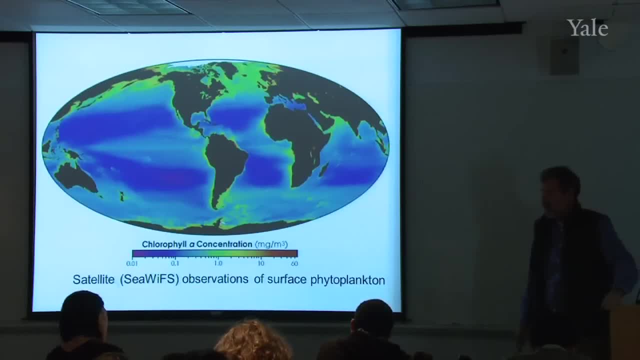 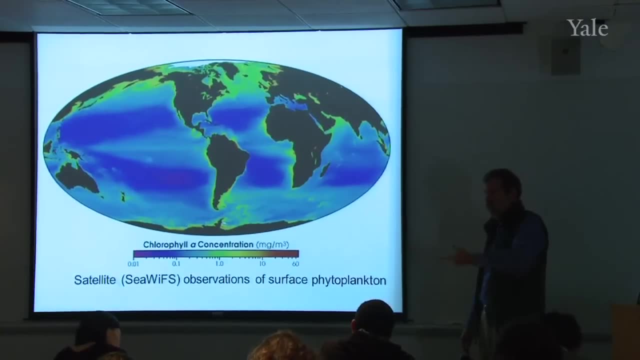 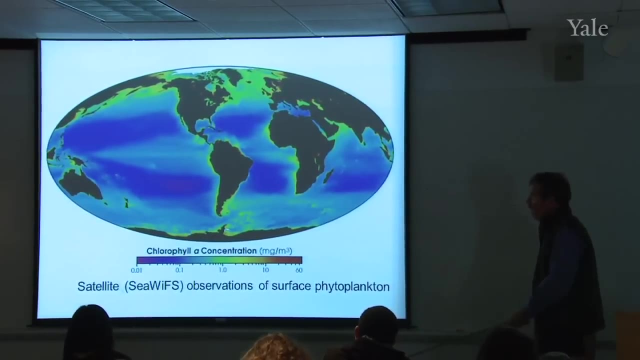 And that's why a lot of the major world fisheries are found in high latitudes, because you can get primary productivity, because you can mix up the nutrient-rich waters into the euphotic zone and get those phytoplankton And that's growing. 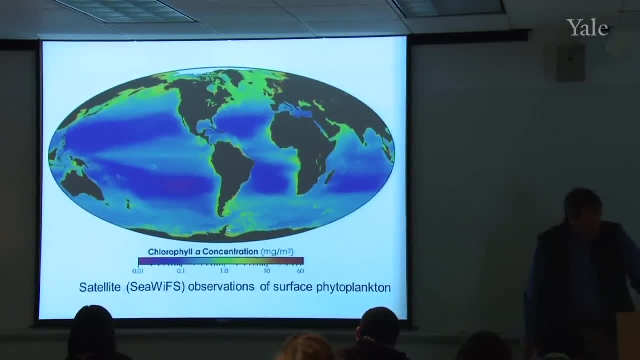 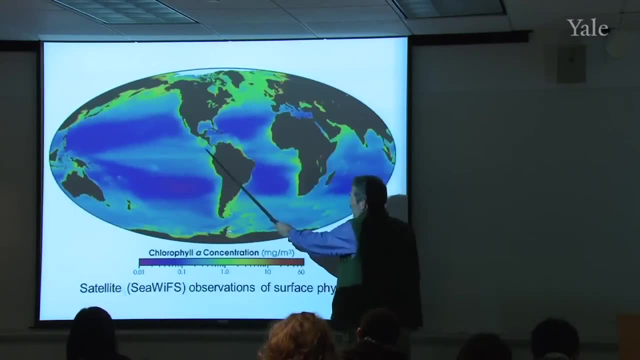 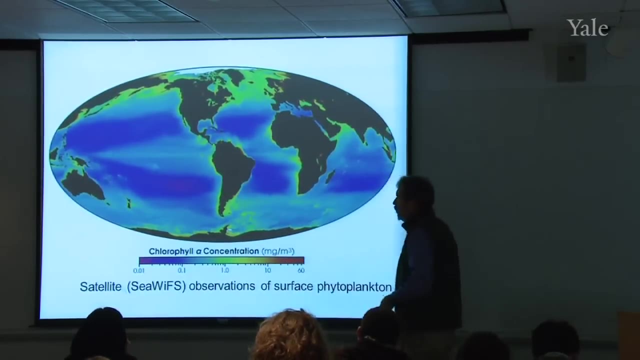 A second example would be- let's see- I'll go back to the order that I had them here- coastal upwelling. There's a lot of upwelling, a lot of productivity, for example, along the Peru coast, And that we believe is due to coastal upwelling. 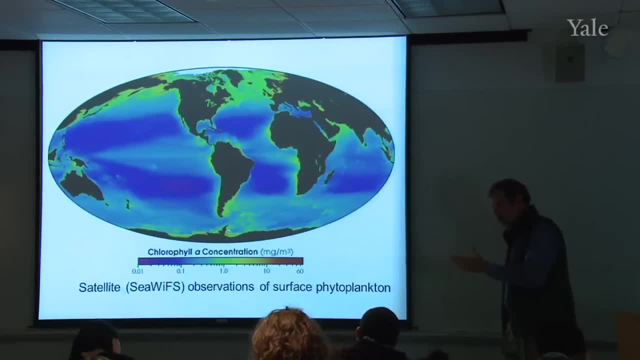 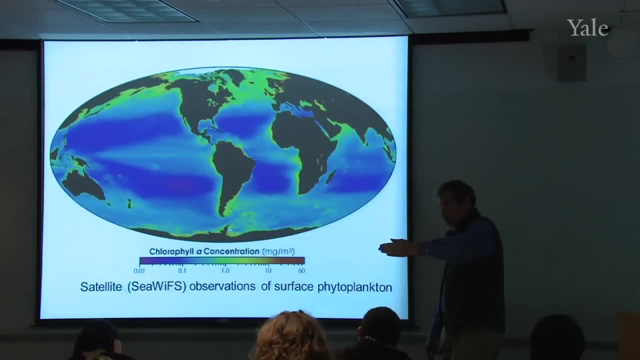 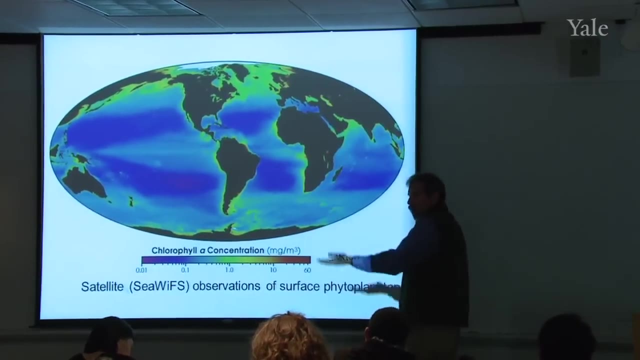 Basically, you have winds putting a wind stress on the ocean and the Ekman drift that responds from that is pushing water offshore. So if you're pushing surface waters away from the shore, then that must be replaced by waters coming up from the deep. 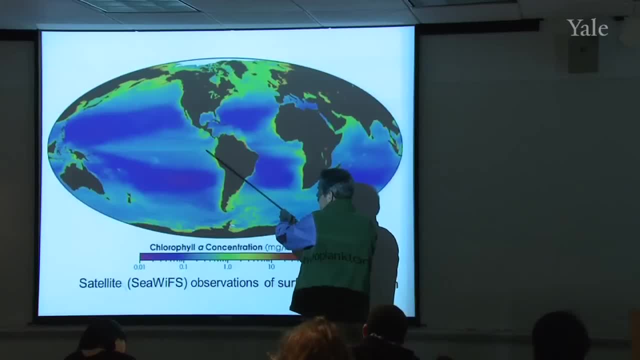 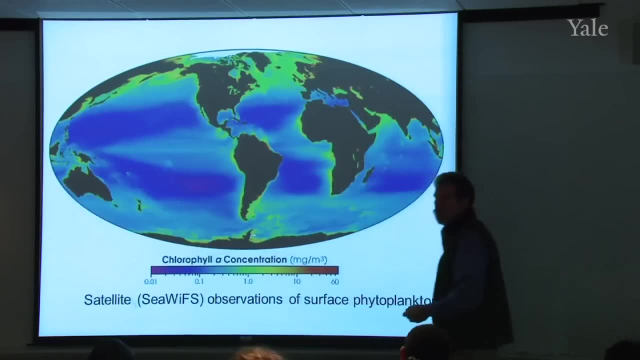 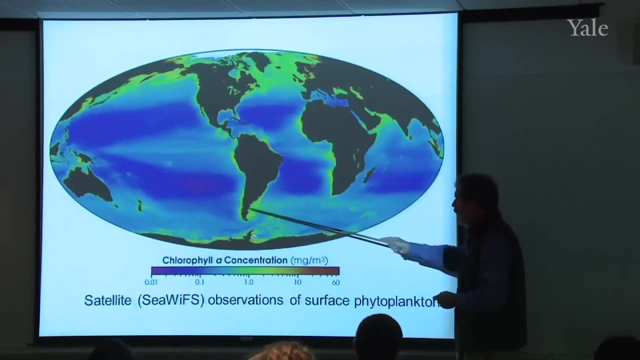 So any time you're, for example, if the wind was like this, the Ekman drift would be perpendicular to that, pushing water offshore and allowing nutrient-rich deep waters to come up from the surface, giving you high productivity along that coastline, And you find that other place. 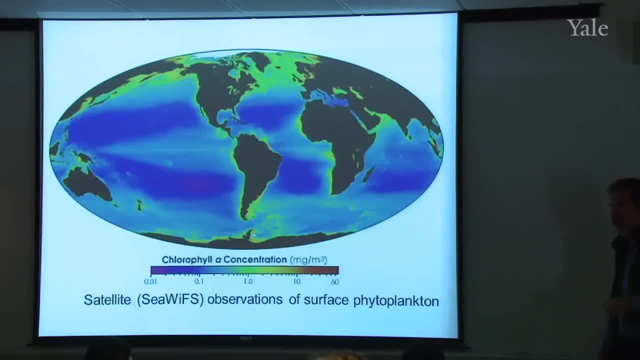 As well. coastlines tend to be highly productive because of the upwelling and the mixing that can occur there: Equatorial upwelling. I think this is the most remarkable aspect of this diagram: is this little line and some other productive. 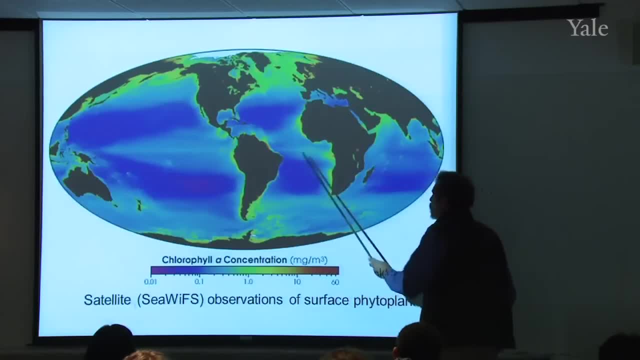 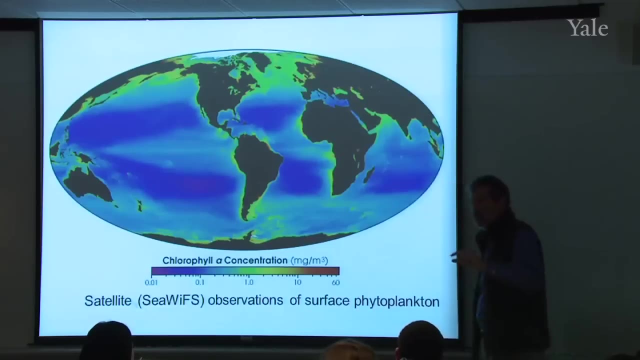 areas around it, but especially that little line right at the geographical equator. That's not at the ice, That's not TCZ, That's not approximately at the equator, That is at zero degrees latitude. There's a highly productive region right at zero degrees. 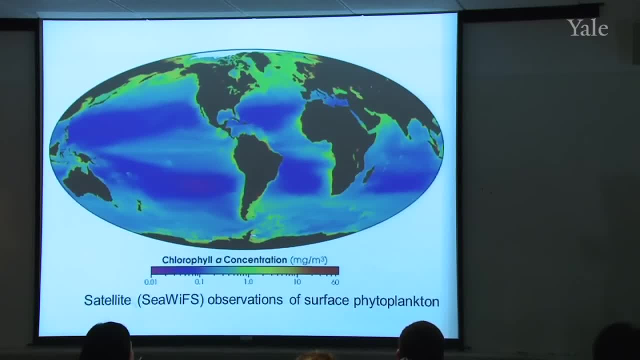 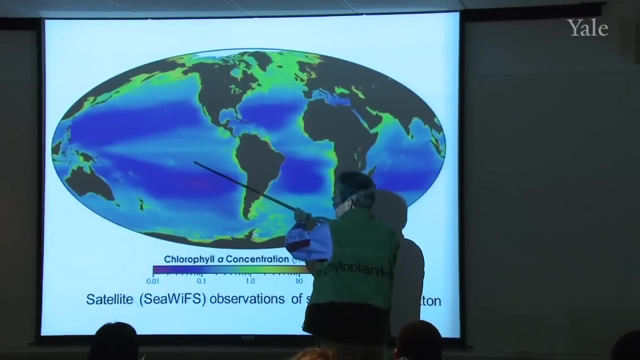 latitudes. And why would that be? Why would there be a highly productive region right at zero degrees latitude? Yeah, A lot of sunlight, but you know the sun, remember? because of the tilt of the Earth, there are seasons of the 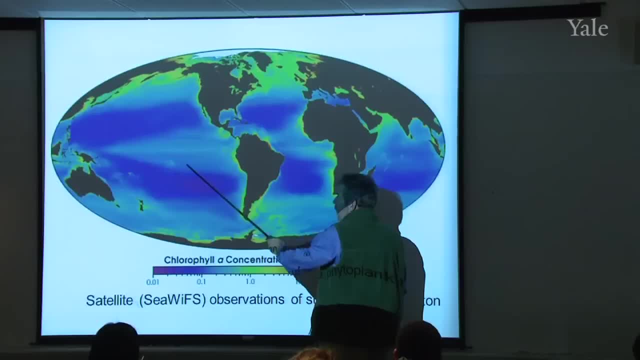 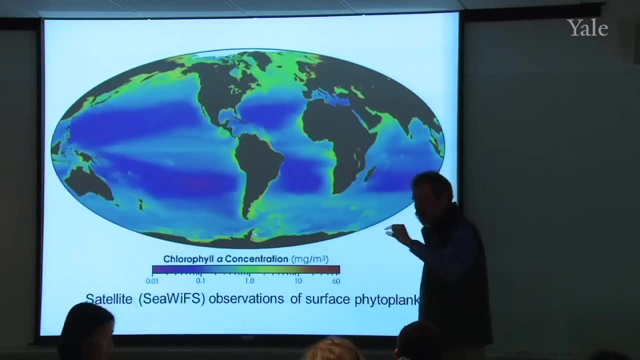 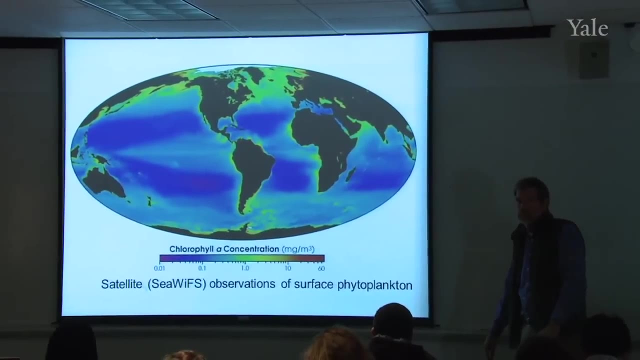 year when you get more sunlight here than there and more sunlight here than there in southern hemisphere summer, And really that begs the question of why it's so narrow. Really, why is it right at the geographical equator? What happens? What's special about the geographical equator? 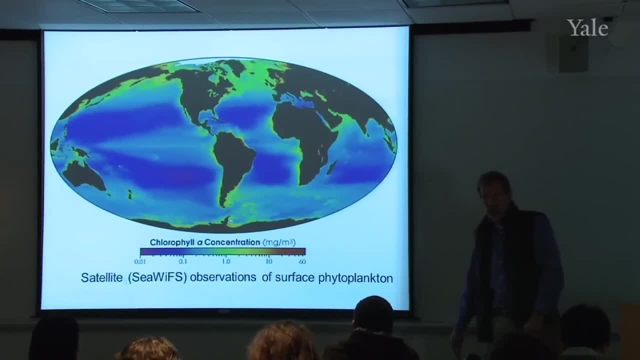 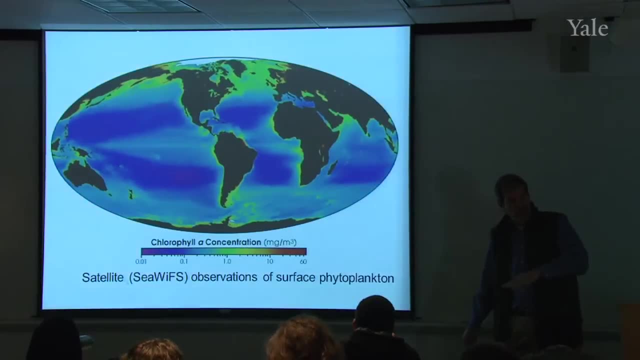 Yeah, North Coriolis Forest And along with that, it's where the Coriolis Forest switches sign from being to the right to the left. That's what's unique about the equator, And I think I have a diagram for that. 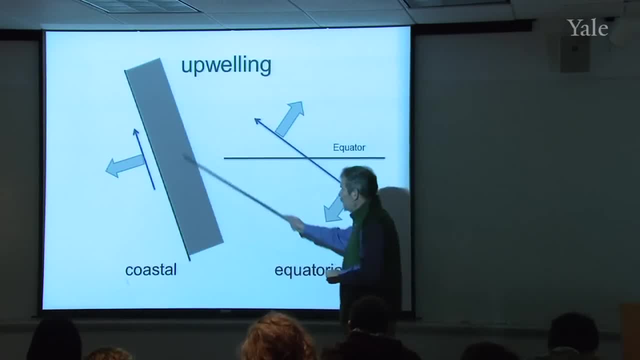 In fact I have two diagrams. So for coastal upwelling, if that's the continent and the wind is like this, it pushes the Ekman drift offshore. it must be replaced by upwelling. Here's the diagram for the equatorial upwelling: 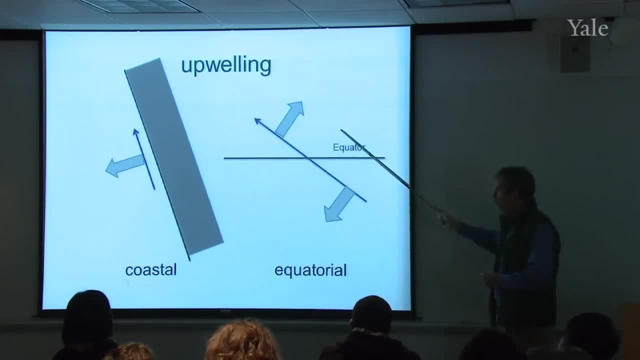 Let's say, the ICZ is located somewhere north of the equator, So the winds cross the equator. The winds crossing the equator are the southeast trade winds, The southeast trade winds. Well, so the wind stress is along the blue arrow. 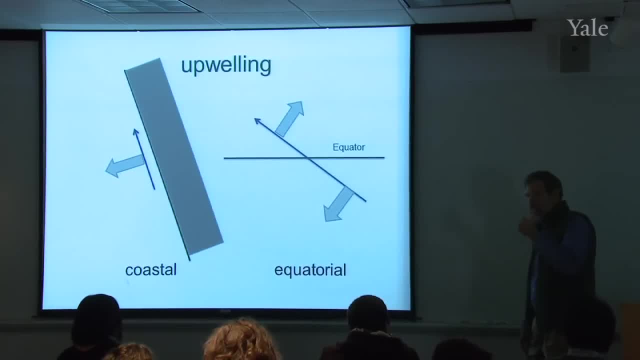 When you're in the southern hemisphere, the Ekman drift is to the left of the wind stress. When you're in the northern hemisphere, the Ekman drift is to the right of the wind stress. So now draw a section like this: That is pulling water northwards, away from the 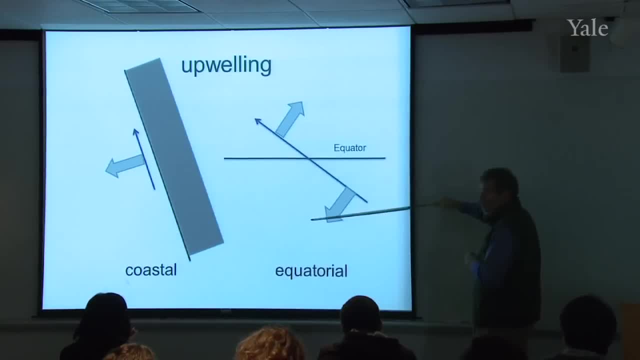 equator. This is pulling water southwards, away from the equator. That water must then be replaced by upwelling. So imagine you're in a bathtub, You put your hands like this, You push water away. Well, that water is going to be replaced from beneath. 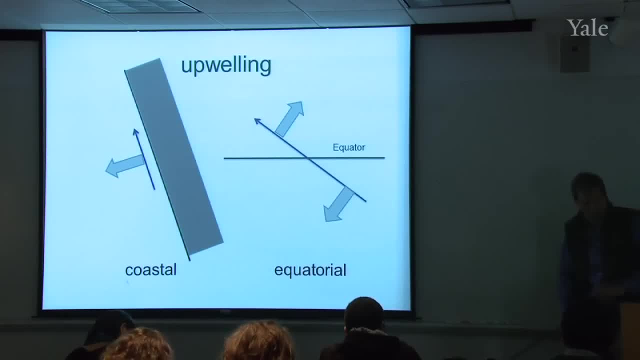 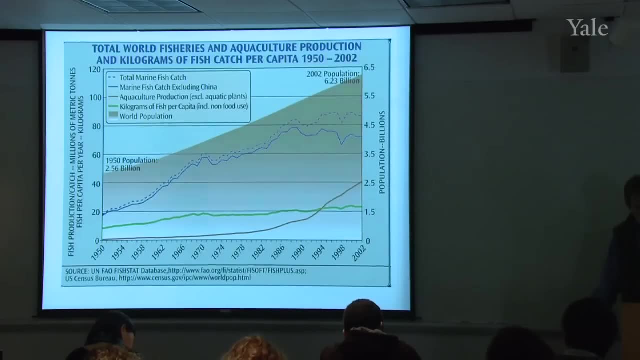 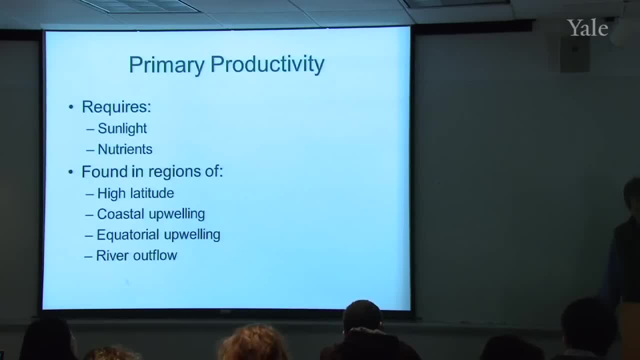 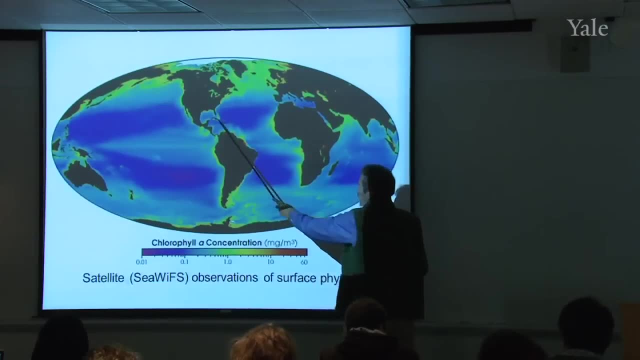 Did I cover them all, by the way? Let's see River outflow. Well, if you look at, for example, where the Amazon River comes in, where the Mississippi comes in, where some of the other major rivers come in, you see, 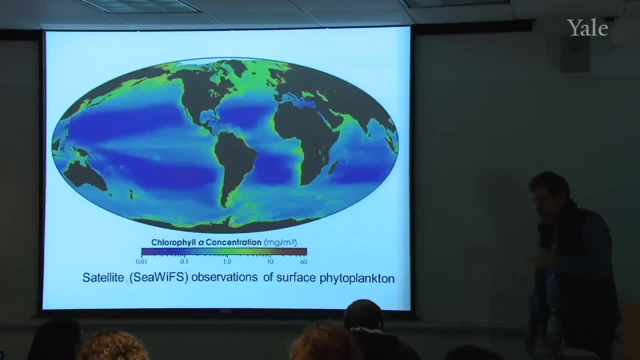 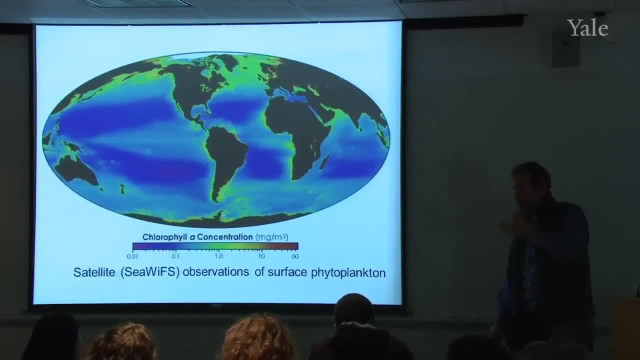 little red regions. That's because nutrients are brought in from the land. The rain has fallen on the land, moved through the soil, picked up nutrients and then, where that passes, that's the out into the ocean. you've brought nutrients into the. 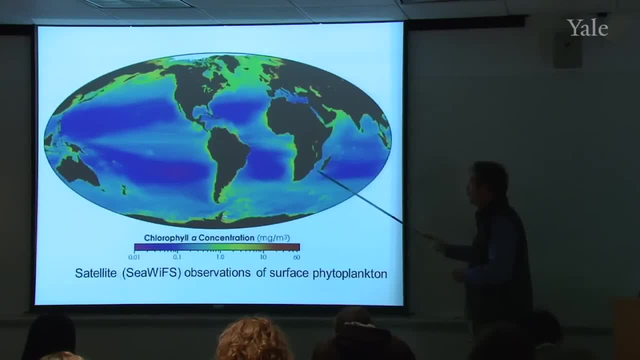 euphotic zone in that way. So that pretty much covers it, why you have high productivity regions in some areas and low productivity regions in other areas. Any questions on this? This, of course, controls. where are the major fisheries? Now it's a little sad to notice that we've pretty much 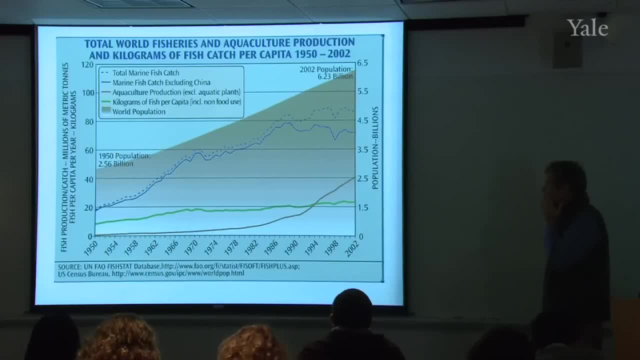 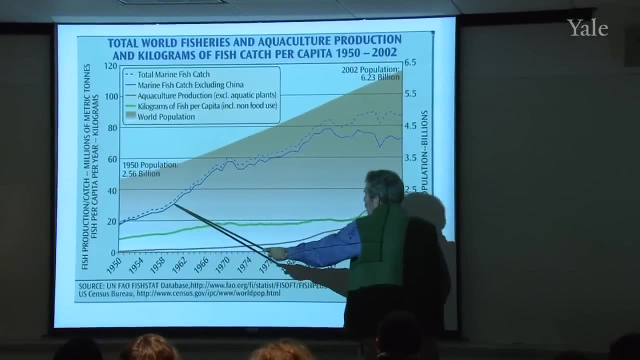 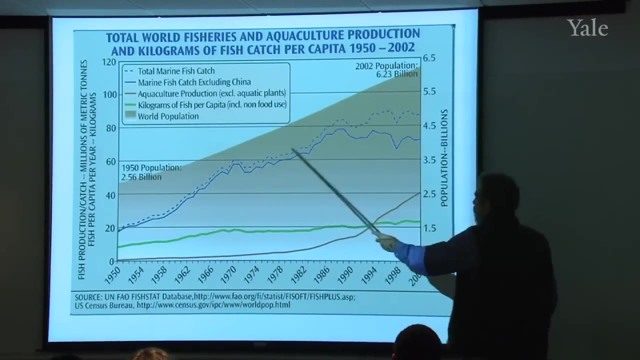 exploited the world's ocean productivity. In the blue is the total marine fish catch from 1950 in units of millions of metric tons, and it's been increasing from the 1950s, But then about 1990 onwards it's pretty much plateaued. 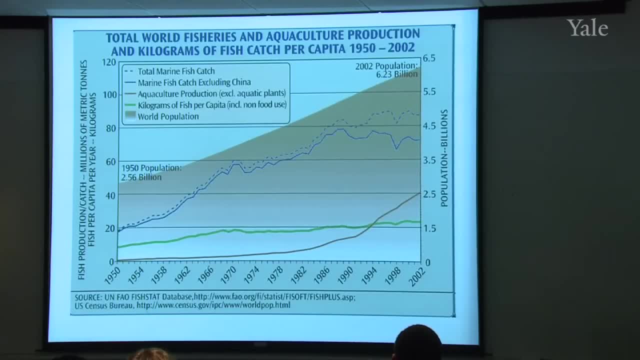 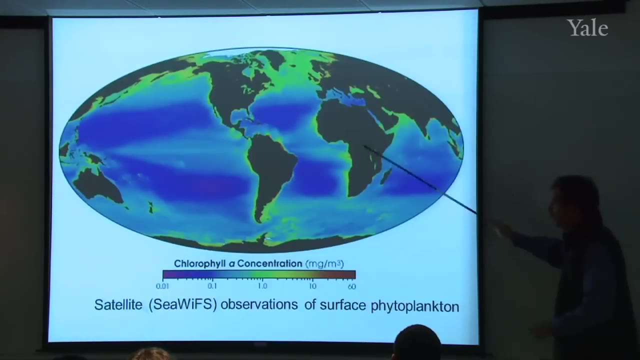 In other words, we're taking about as much edible biomass out of the oceans as the oceans can produce. So the human population has grown To the state that it's pretty much fully utilizing everything that the ocean is producing in these high productivity zones.